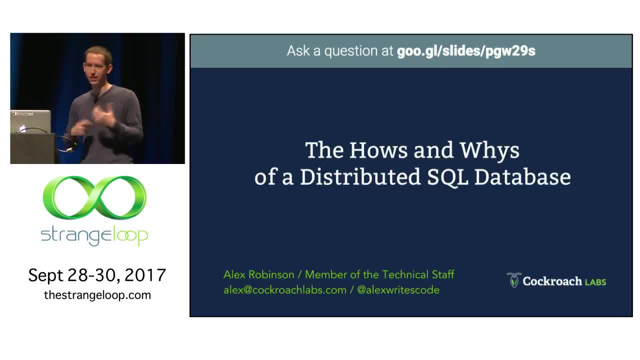 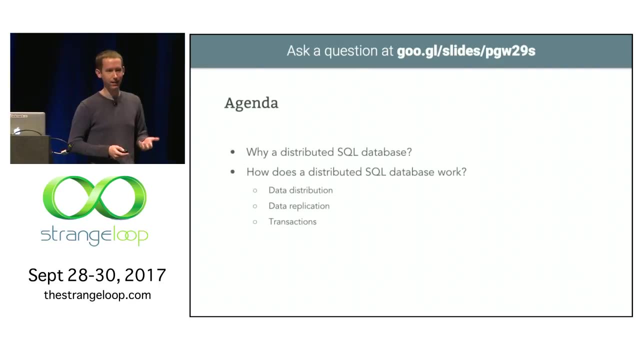 these distributed SQL databases. I'm interested in how they fit into the historical context of databases, why they're being built now as opposed to 20 years ago and what makes them different from old databases. Thank you, And so that is what we're going to take a look at today. You know why a distributed 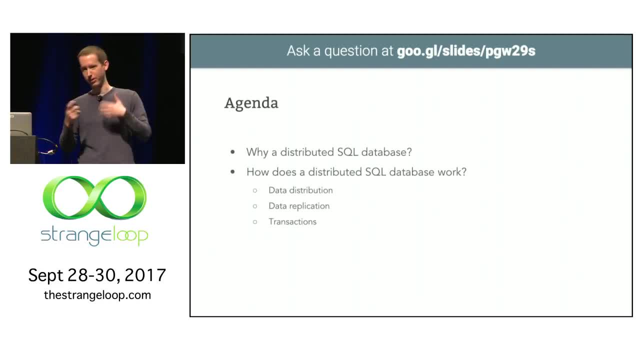 SQL database. Why would anyone care about them? Why would you devote years of your life to building these things or millions of dollars to building them? And how do they work? So specifically in the how they work, we'll look at how data gets spread around the system. 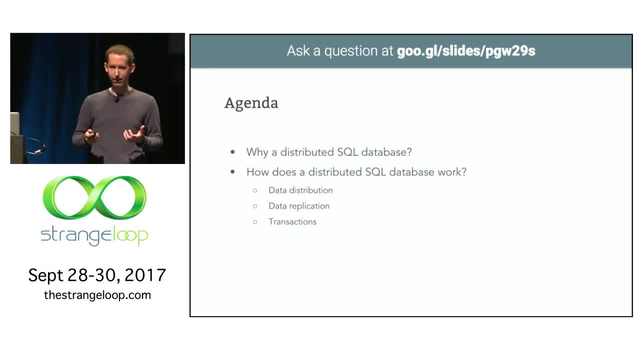 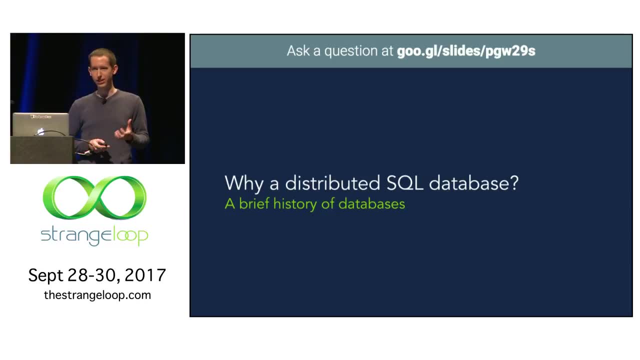 how it gets replicated in a consistent way, and then how transactions get layered on top in this distributed computing environment. And so let's start by looking at the history of the system. Any time someone introduces a new system, you really need to ask why, How. 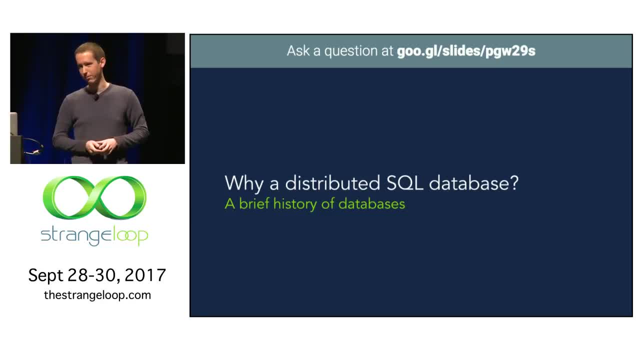 is this system going to be better than the hundreds of systems that have come before it in the history of computing, And why is it being built now instead of previously? What do you know now that developers before you didn't, that they weren't able to build? 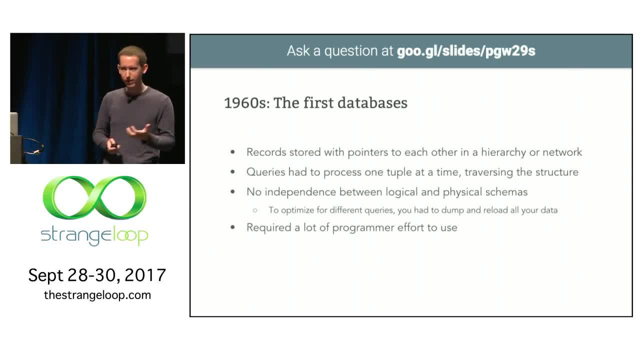 the system instead. And so we'll begin with the very first databases, And these were being built in the early 1960s at companies like IBM and General Electric. These databases were pretty primitive. They were the first ones of their kind. They didn't know a whole lot about what they were. 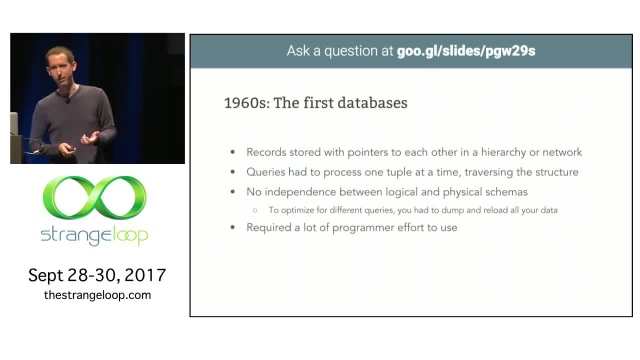 doing. yet The interfaces that they exposed to programmers were very tough to use. So, rather than having, like, a table of records like we're used to today, or a key value interface, like we're used to today, it was almost like they were programming more against an in-memory. 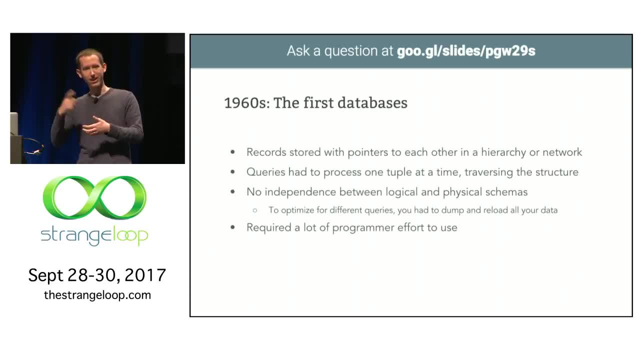 data structure. There were these series of records that your queries would have to iterate over one by one and traverse links between the records. So you might traverse from, like, an organization record to iterate over all of the employee data And you might have to iterate over all of the employee records that are working at that organization. 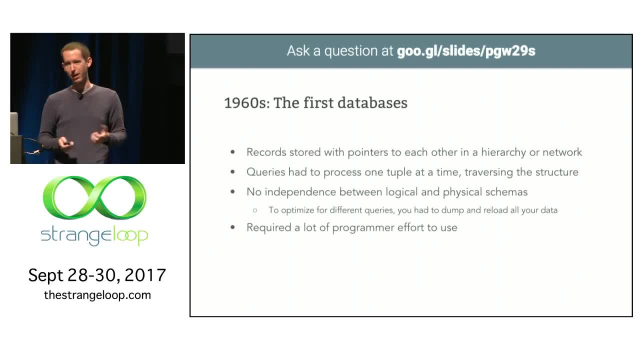 And the queries that you wrote were really tightly coupled to the storage format of the data on disk, And so if you ever wanted to change that to optimize for different access patterns, you'd have to pull all the data out of the system, load it all back in and 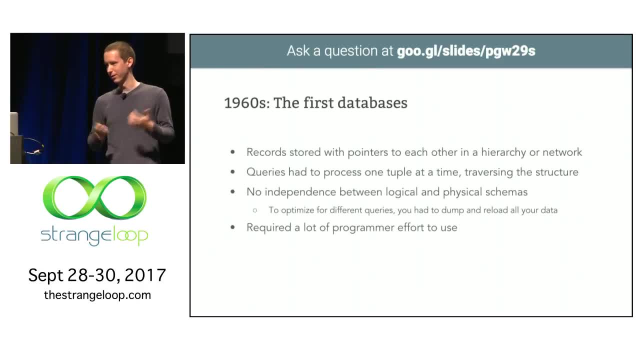 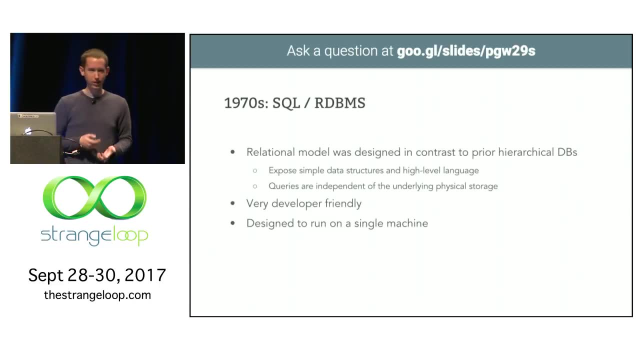 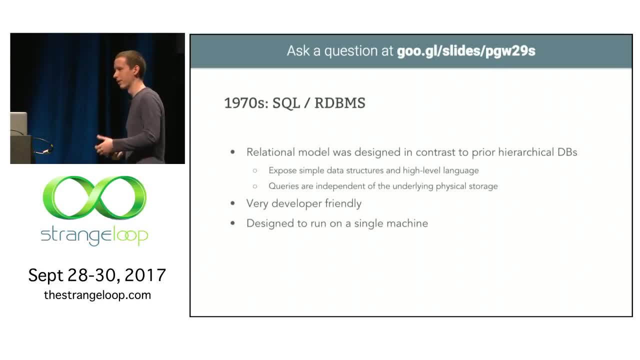 to do this, I'm going to do this, I'm going to do this, I'm going to do this. And so he had a lot of the programmers around him at IBM in his office having to spend a ton of their time rewriting these queries: optimizing the access patterns, changing the layout of 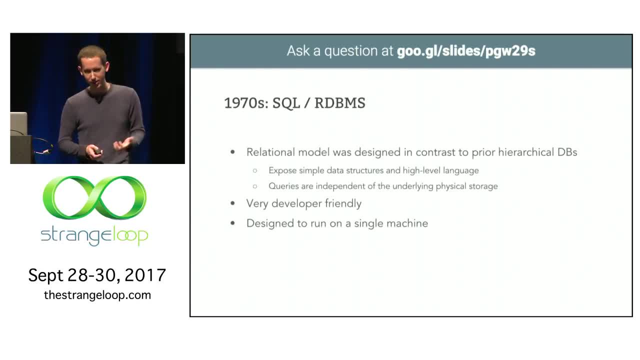 data on disk and thought that there had to be a better way. And, being a mathematician, he was all about elegance, And so he created what's now known as the relational model, which powers all the SQL databases you're familiar with today. And this relational model. 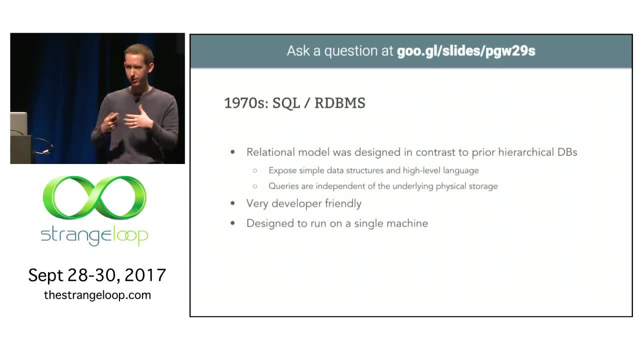 wanted to get rid of this tight coupling between queries and how data is stored on disk, So it relies on very simple data structures, the table that you're probably familiar with, and a high-level query language, which is now known as SQL, And the queries here are: very independent from the storage on disk. So the database software is free to optimize things underneath the covers without the programmer needing to worry about it. It can change how things are stored without anyone ever having to know. So these systems were much more developer-friendly. And, as a note of historical context, they were always designed to just run on one machine. In the 70s, most organizations didn't even have one computer, let alone multiple computers, let alone have multiple computers that they wanted to devote to. 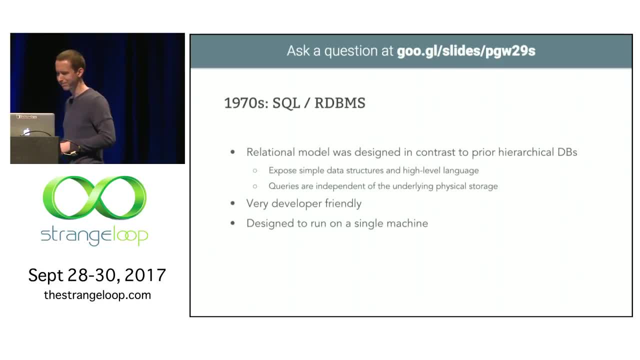 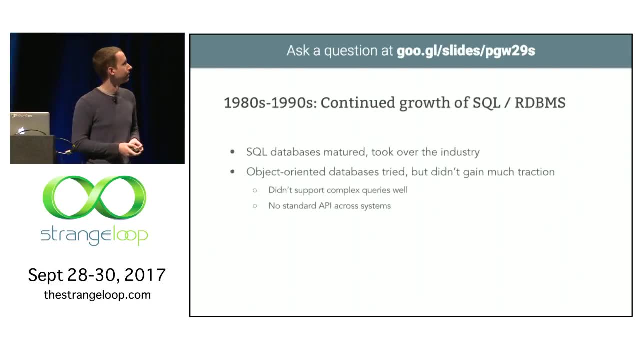 So these systems were always built for a single machine. The first commercial database was released in 1978 by Oracle and it just kind of exploded from there. Over the next couple of decades, SQL continued to mature, to grow, to gain popularity. More vendors started putting 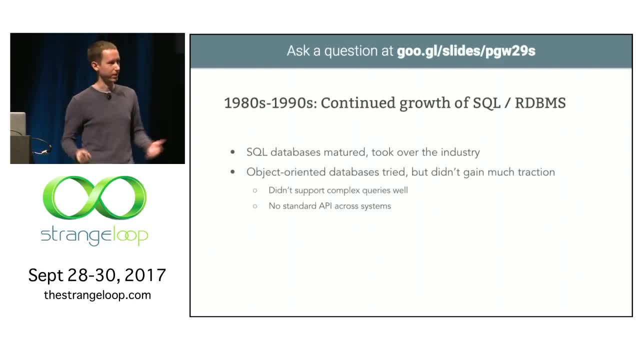 out SQL databases. There were acquisitions, There was lots of competition. It was great. But in this time there was also a new kind of database that got introduced. that didn't really take off. You know, it was attempted but didn't get the necessary training. So 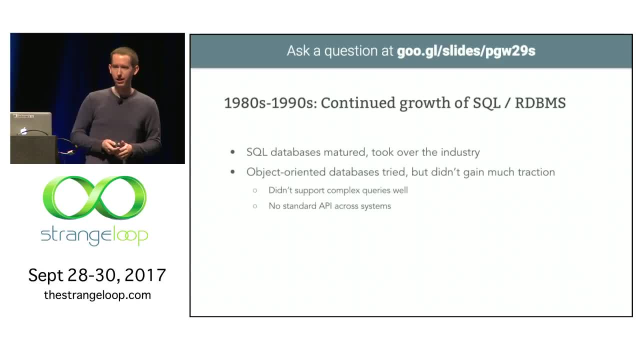 it was a great attraction, And these were object-oriented databases. The motivation for these systems was that object-oriented programming languages were growing in popularity in the 80s as well- C++, I believe, Java- And there is a bit of an impotence mismatch. 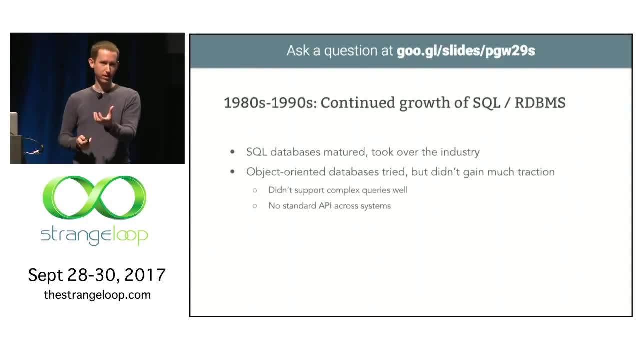 when you're trying to translate between the objects that your program has in memory and the rows and columns that SQL databases store. So they argued that these were easier to use because you could effectively just take an object in memory and dump it into the database as a single object. 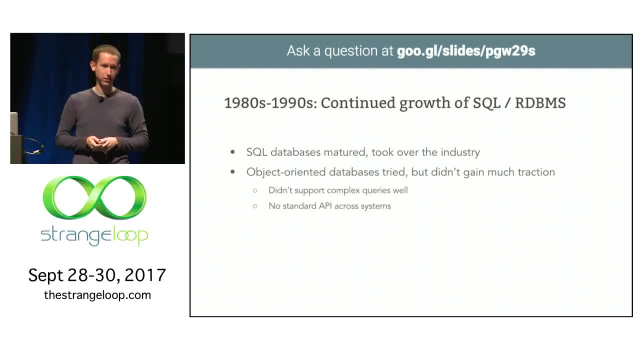 It was a lot like today's document-oriented NoSQL databases, But at the time there wasn't enough reason to switch. In order to switch, you had to give up things like complex queries that SQL databases allowed And all these different object-oriented databases had pretty. 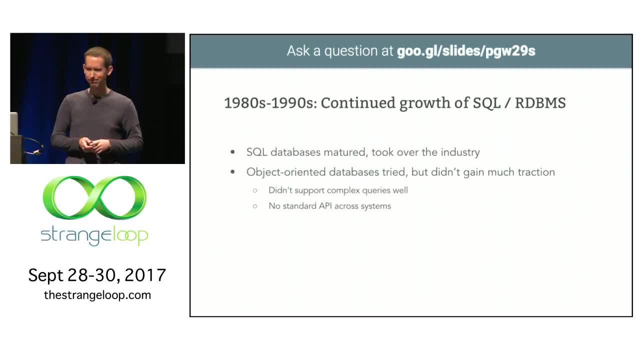 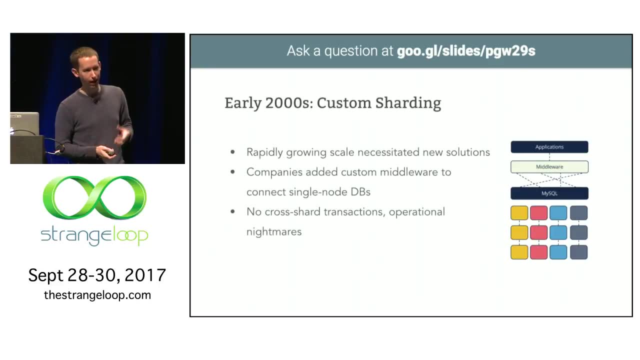 disparate APIs. There was no real standard, as there was with SQL, So these systems never quite took off. The first real big change in how databases worked or how they were used came in the early 2000s during the Web boom. Suddenly there were more and more companies that needed to support more and more users. 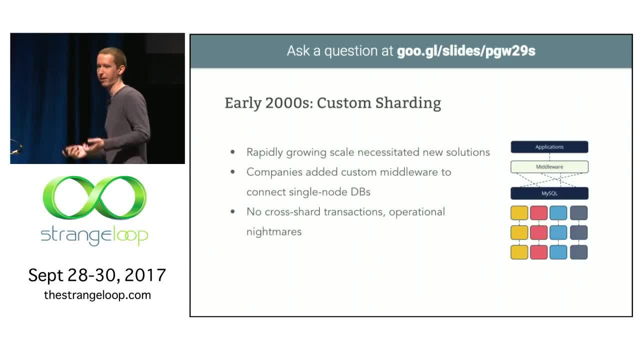 They had to build services to support millions and millions of users and it had to be up 24-7. And they just couldn't scale their databases to support this. You can only scale a SQL database as big as you can buy a single machine. So you had these big web scale companies like 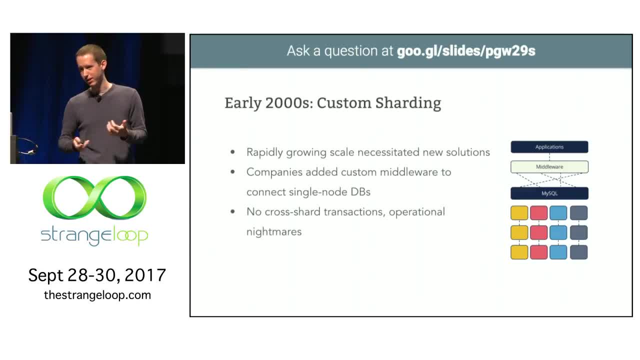 Google, eBay, Yahoo and Amazon all having to deal with things like sharding their database, And what this really meant was just that they'd get 10 machines to put their data on and they'd break their table up into chunks, So the first chunk would go on the first machine. 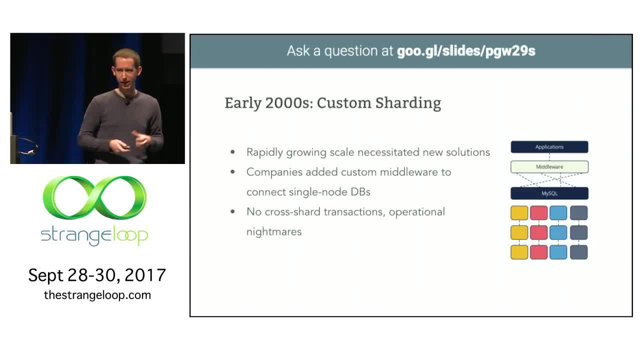 Second chunk would go on the second machine and so on. So this all had to be done manually by a database administrator, And then for queries to work they had to put this middleware layer in front of all these shards to translate application queries into separate queries. 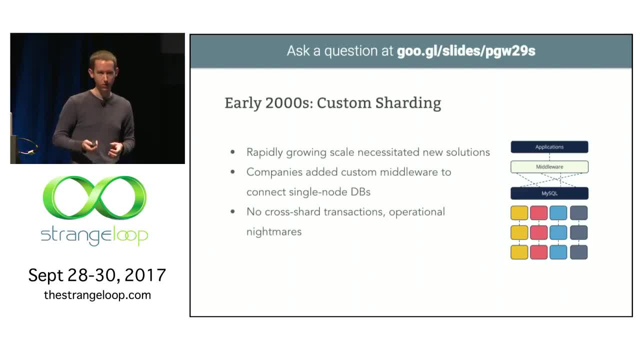 for the separate shards. This limited what programmers could do because they couldn't really do things across shards And any time the data grew to be too big to fit on their current number of shards, it was a huge operational headache to try and reshard to move all the. 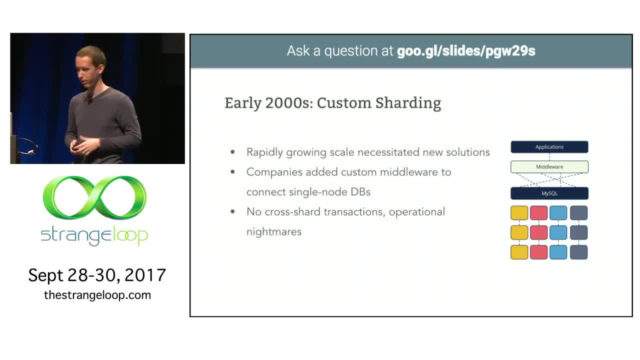 data onto different machines So you could have more of them to account for all the growth, And so this was worth it for the really valuable services that these companies were building. back then, Like Google, famously sharded a MySQL setup for their AdWords product, But they realized it wasn't worth. 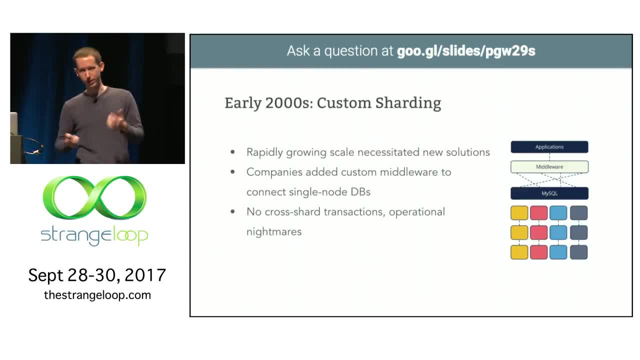 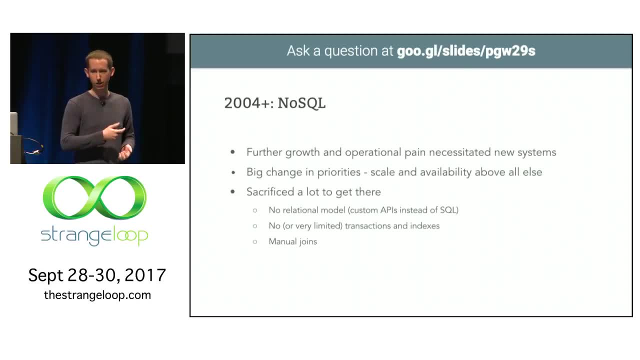 it to do this for all the little services that they were building. This might not be worth it for smaller services like Google Calendar, due to all the effort involved. And so, around this same time, those same companies- Google, Facebook, Amazon- all started building. 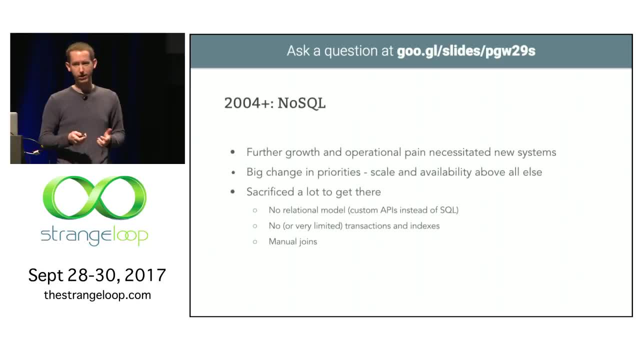 databases, And these NoSQL databases had the primary goal of being scalable. They wanted scalability at pretty much any cost because they needed to build bigger and bigger services and continue scaling as they knew more and more users would be coming online over time. So these NoSQL systems had to give up a lot of things in order to get the scalability. 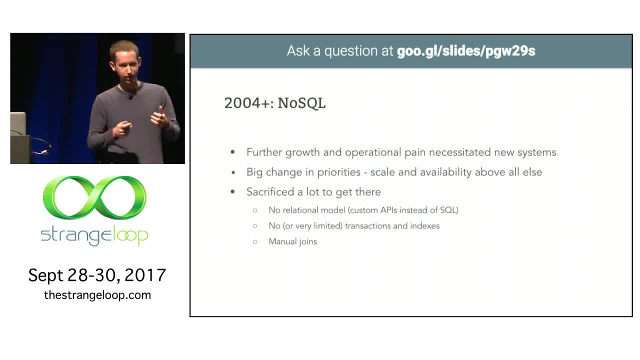 that they were after They gave up the relational model. Obviously, that's why they're called NoSQL, which is kind of a silly way to define a class of systems due to what they're lacking. But they're called NoSQL databases And they also gave up things like transactions and 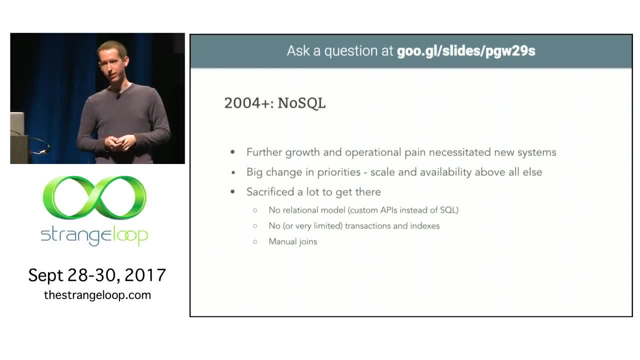 joins and indexes. for the most part, They usually didn't offer the same sorts of consistency of data that programmers were used to with SQL systems. And so you know, whereas TedCod in the 70s took complexity out of users' applications and brought it into the database to make life easier for developers, NoSQL systems did the. 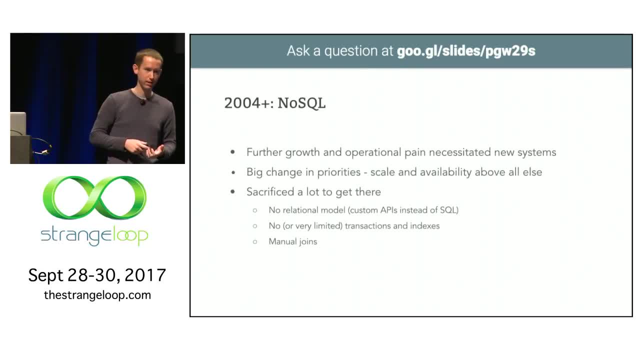 reverse. So they took the complexity that had been built into the database to make life easier for developers and just pushed it back out into the applications, saying like, oh, we can't handle this anymore, You're going to have to deal with this, You're going to 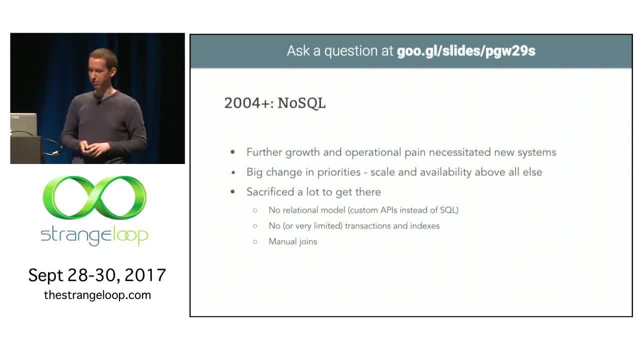 have to work around the database's- insufficient capabilities. And so now we're in the 2010s and there's this new class of systems coming around, sometimes called NewSQL, or you can call it Distributed SQL. Some people call them Elastic SQL, whatever. 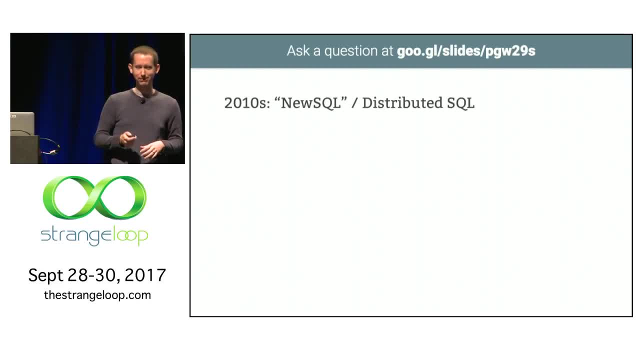 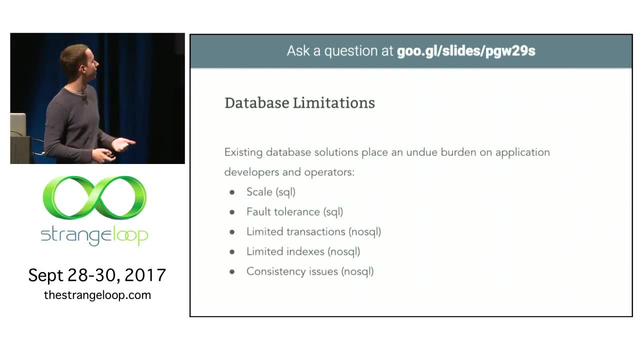 the heck you want to call them. They're SQL databases that run on multiple machines. And why are these being built? I think it should be fairly clear at this point, based on the history. But without NoSQL or without Distributed SQL, you have to make a choice. when you're starting a new product, Are you going to pick a SQL? 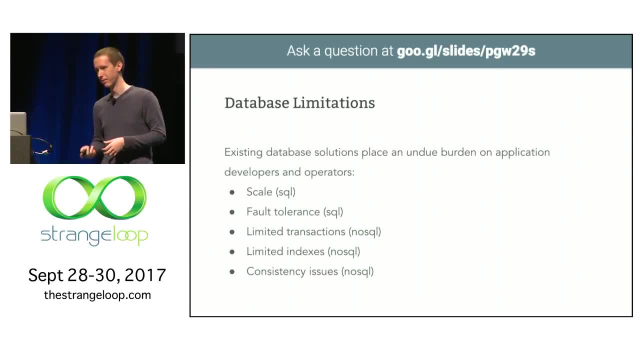 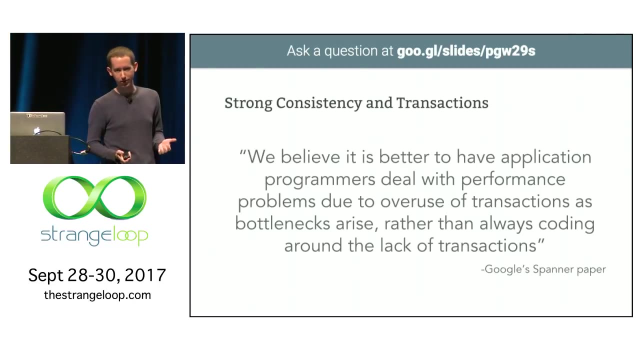 database and limit your future scalability? Or are you going to pick a NoSQL database and take on an extra development burden to work around the lack of a solid foundation to build on, Because the NoSQL systems don't have transactions and indexes and consistency in general And there have been a lot of really successful services built on top of NoSQL? 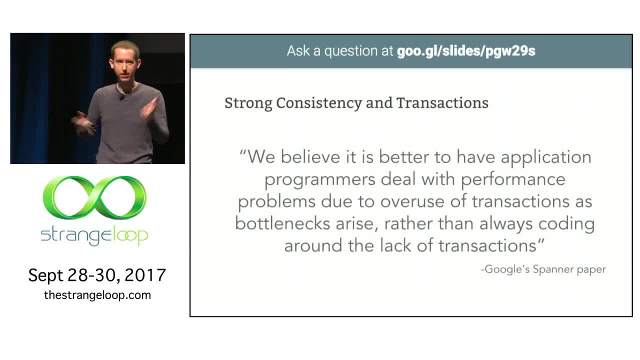 databases right, So they're clearly not completely useless. Tons of great services have been built on top of them, But it's a lot harder, And so Google, who published a paper about their Distributed SQL database, which is called Spanner, back in 2012,, put in this choice. quote about why. they thought it was worth it to build this system and to have most of their services switch over to using it, And they think it's more worthwhile to have their developers occasionally deal with performance problems than to always have to deal with the lack of transactions. 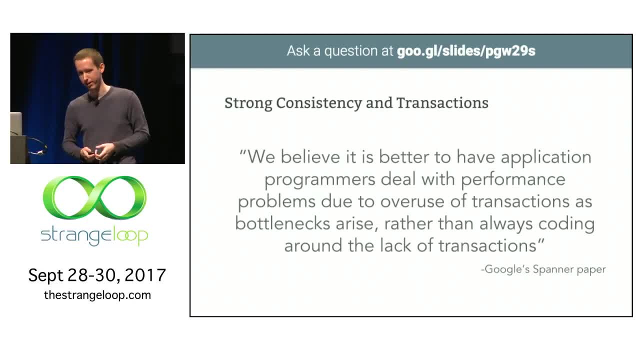 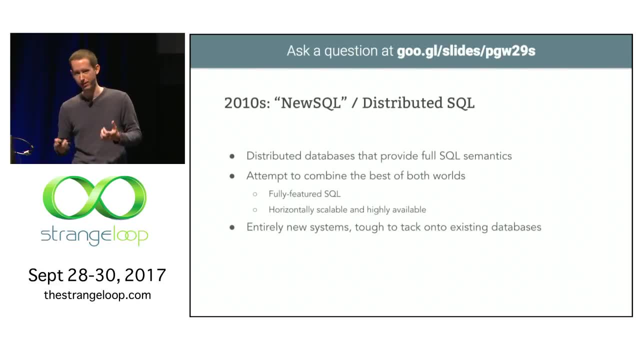 It saves Google money in the long run to do this, because it saves their developers time and energy, And so that's why these systems are being built, Because we want to try to eliminate that tradeoff that was inherent in picking a database five to ten years ago. So there's a whole class of these systems appearing that are 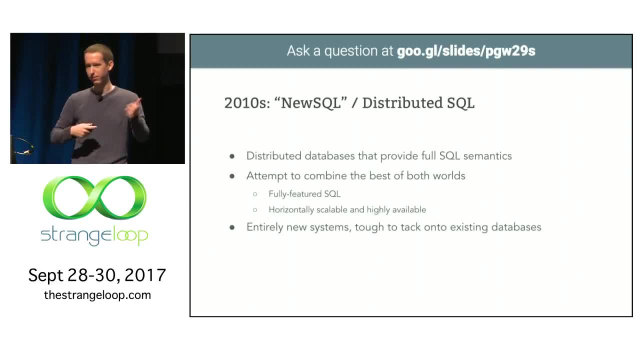 distributed databases providing full SQL semantics where you can go and talk to any of the machines in the cluster as if they're an individual node, but they'll do all the coordination under the covers to work together as a distributed system to process your queries. And so we're. 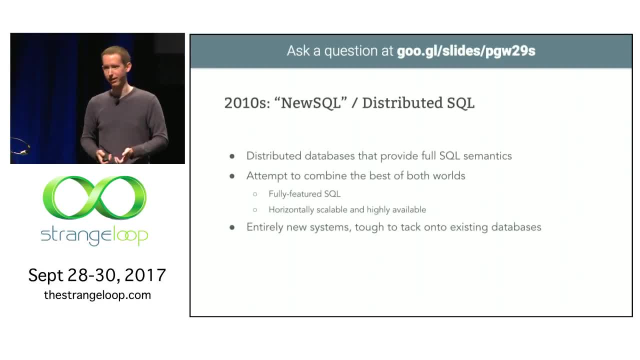 attempting to combine the best of both worlds, And these are usually built as entirely new systems, because to build this functionality into a previous database you basically have to rip out the guts and put in entirely new guts, like an entirely new engine, And at 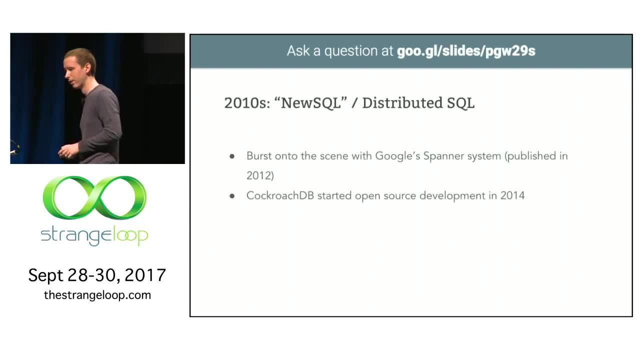 that point it's almost like building a new system anyways. So the two primary systems I'm going to be referencing a lot today, just because I'm most familiar with them, are Google Spanner, which was published back in 2012 and had another 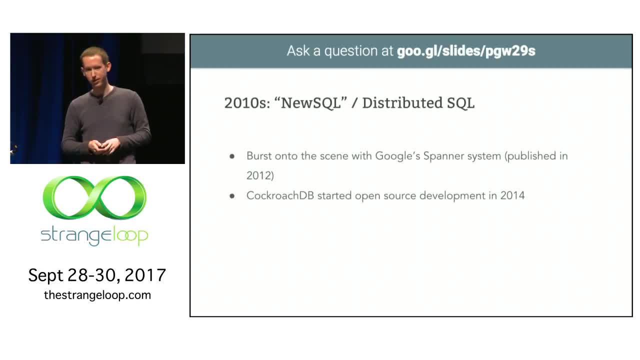 paper published earlier this year detailing how it's changed in the years since. and then CockroachDB, which is because I work on it on a daily basis And all the information is publicly available out there on the internet due to it being open source. So that's why. 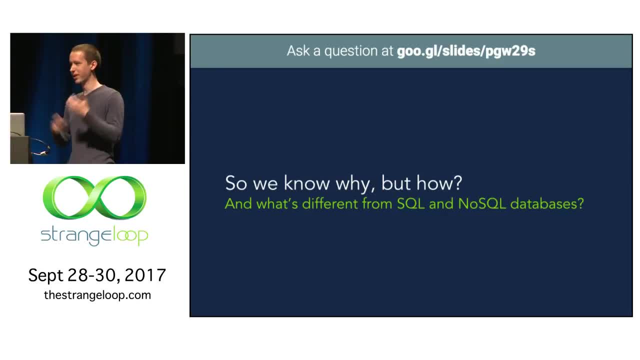 these systems are being built. So let's look at the system, and I'm going to talk a little bit about the system itself, But there's still the question of how. So what makes them different? Why couldn't they have been built 20 years ago? And how are they getting this different set of trade-offs? 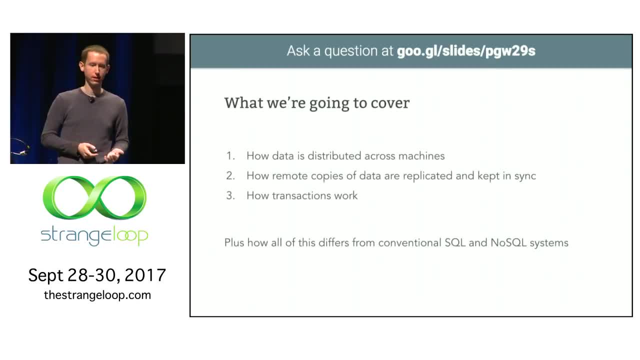 So we're going to specifically focus on, as I mentioned earlier, how that data is distributed, how remote copies of the same data are kept in sync in a way that keeps it consistent, and how transactions work in the distributed setting, And for each of these points, I'm going to specifically compare all the different types. 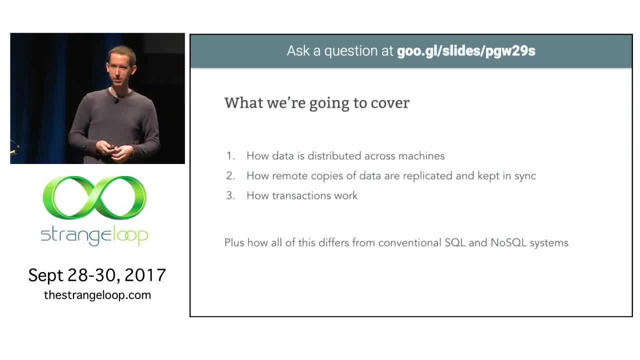 of databases, so how SQL databases do things, how NoSQL databases do things and how these new SQL or distributed SQL systems do things. As a brief disclaimer, there are a ton of databases out there that work in different ways. So there's a lot of SQL databases. there's a lot of NoSQL databases. I can't 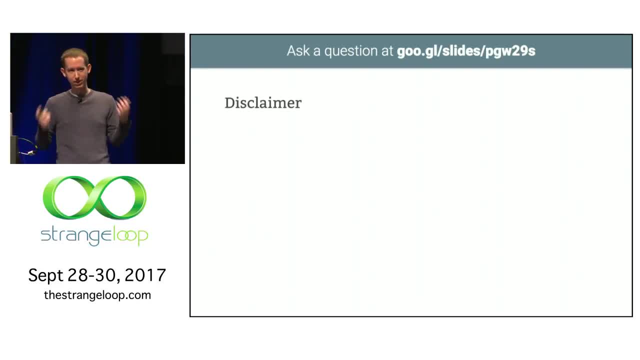 cover every little exception to every rule. I'll do my best to speak in generalizations that are as true as possible and point out exceptions where there are some, but there are too many systems for me to know all of them, let alone to point out all the differences. 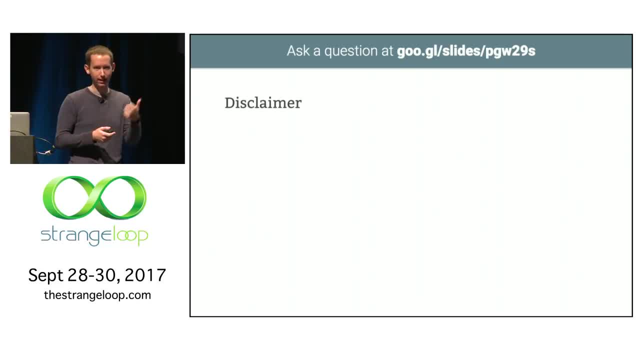 today And, as I said, I'm going to be focusing mostly on Spanner and Cockroach as representative of new SQL systems. So let's dive into data distribution. All the data distribution means is just this question of how we're distributing data amongst the cluster, And for SQL databases there's 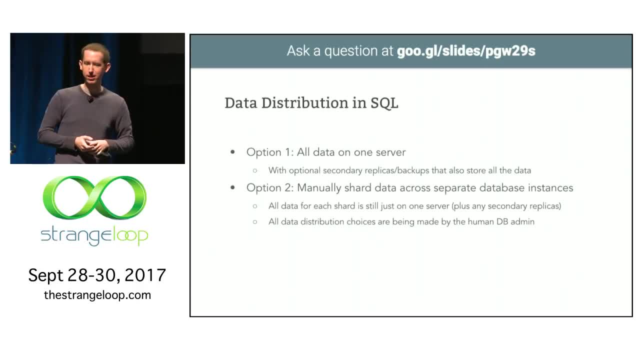 not a whole lot to talk about because they're designed to run on a single machine, right? So all the data is on your one server And you might have backups somewhere. you might have secondary replicas that are getting copies of the data you know in a streaming fashion. 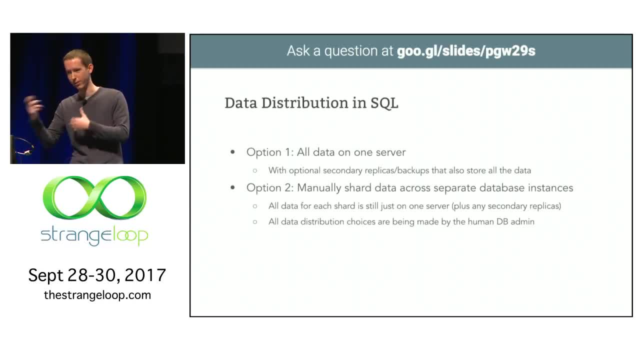 right, But all the data is on one machine or all the data is copied onto a couple machines. There is this option, as I mentioned, to manually shard data across multiple instances of a database, but that's not the database software doing anything. That's still just the database. 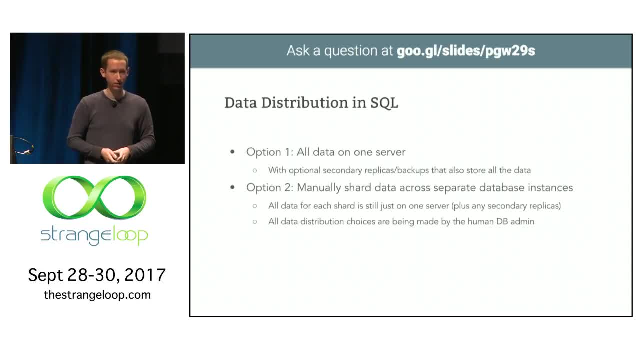 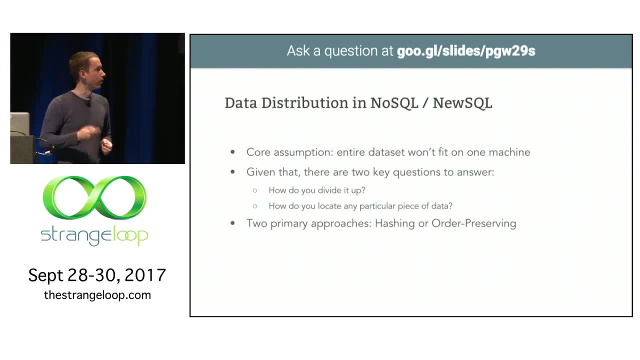 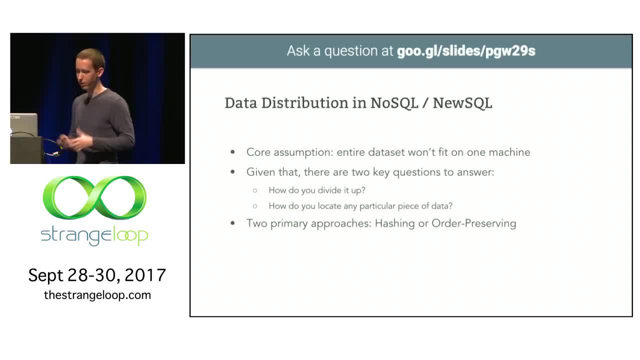 do that. You can't do that. So there's this core assumption. that means you're going to have to break up your data in some way and divide it up amongst all the machines in your cluster. So NoSQL really pioneered some of these techniques, And new SQL has effectively. 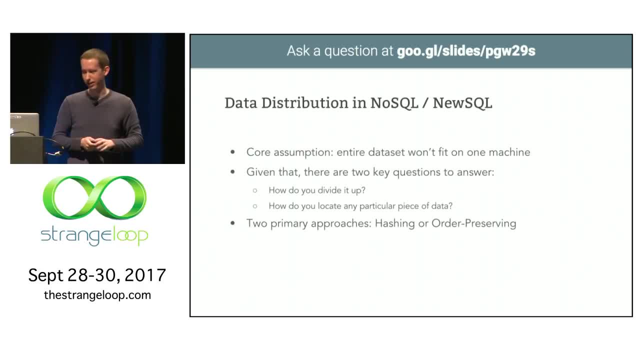 just learned from them saying: you know, NoSQL did this well, We have no reason to change it. Let's keep doing things in a similar way. And so you have to answer for all these systems, how you divide up the data into chunks, And 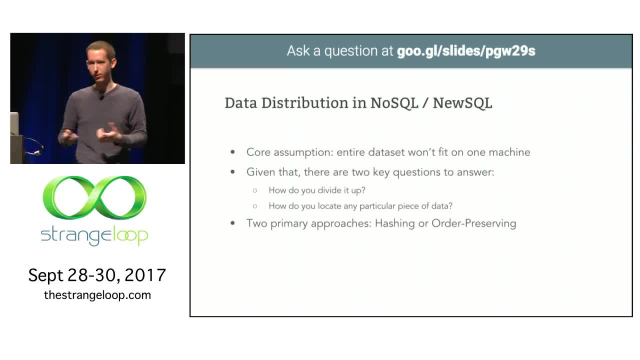 then, once you've divided it up, how do you find where those chunks are located within the cluster? it's no use to have your data broken up and spread out if you don't know where each piece of data actually is at any given time. 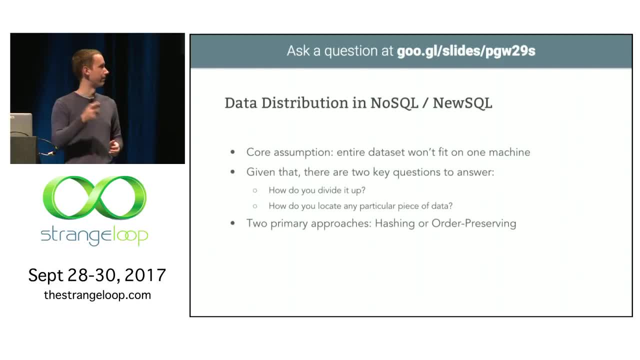 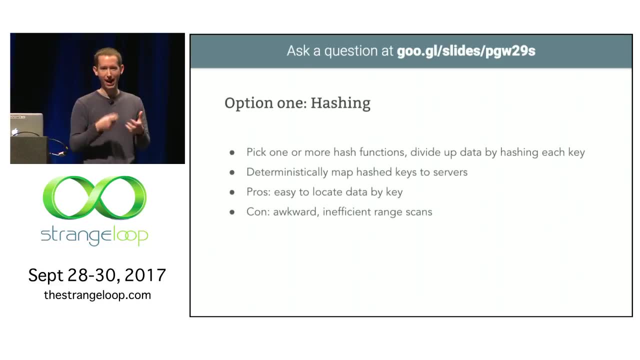 There are two primary approaches to doing this, which we'll take a look at individually: hashing and order preserving. So this hashing approach to data distribution just means that you're going to pick a hash function, maybe multiple hash functions, and you run these hash functions on the keys. 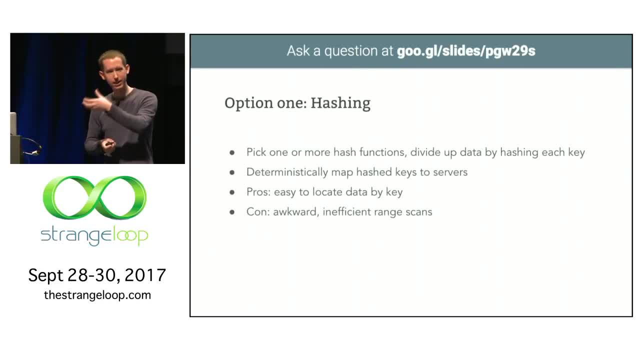 assuming it's like a key value system. So you run the hash function on the key, it spits out a result and you deterministically map that result onto one of the machines in the cluster, Maybe just by doing a modulus on the number of machines or something along those lines. 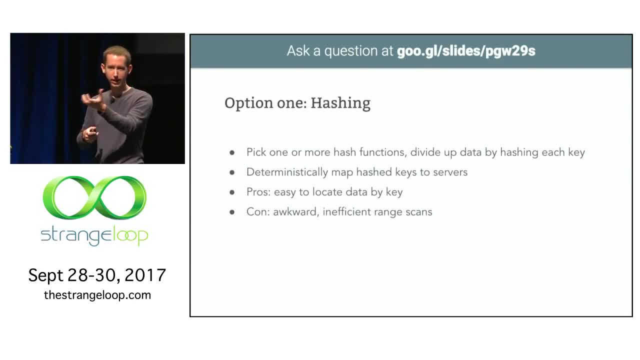 And this makes it super easy to find any piece of data, because all you need to do is run a function on this key and you know exactly which machine or which machines it's going to be located on. So reads and writes can find the given machine they want to talk to really quickly. The problem here that makes this prohibitive for new SQL databases is that you can't do range scans because hash functions don't maintain ordering of your data. So if you wanted to do a hash function, you'd have to do a hash function. 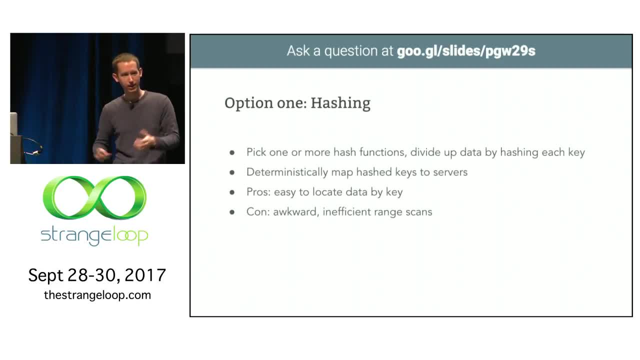 If you wanted to scan over all the keys from A to B. you can't do that efficiently in a system that's dividing up the data based on a hash function, So this approach is used in databases like Amazon's DynamoDB or in Cassandra by default. 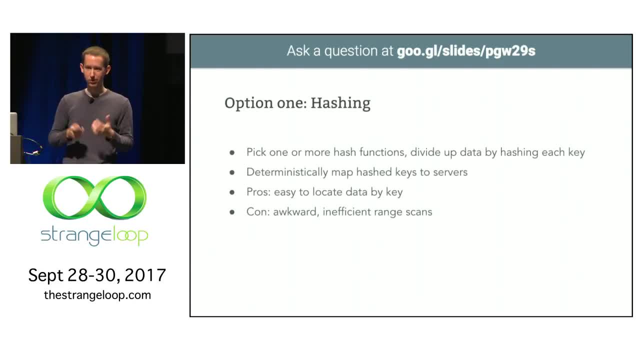 but it's not used in any new SQL databases as far as I'm aware, because SQL databases really rely on having ordered indexes in order to access data efficiently. So some other NoSQL systems like Bigtable and HBase, as well as most new SQL systems, 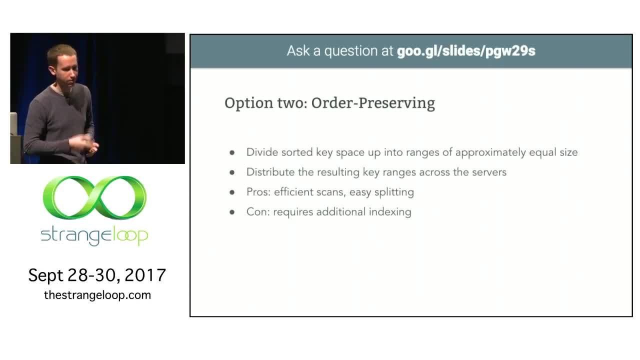 I know of use what's known as an order problem, And this approach means that you put all your data, lay it out from A to Z or from the beginning of the alphabet to the end of the alphabet, in alphabetical order, and just 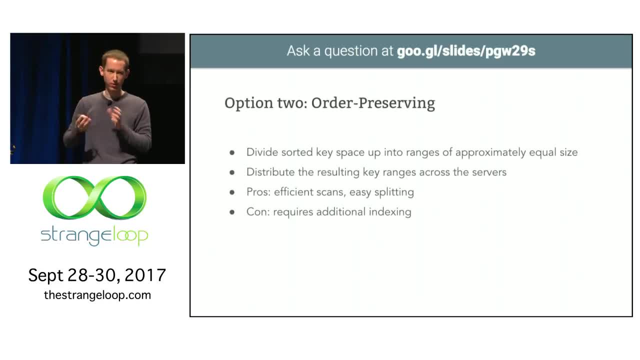 split it up into chunks by picking arbitrary dividing lines that give you nicely sized chunks in the middle. So you might have a chunk from the beginning of the alphabet, through A, from A through F, from F through Q and so on, And you just distribute these chunks evenly across all the nodes in the cluster. 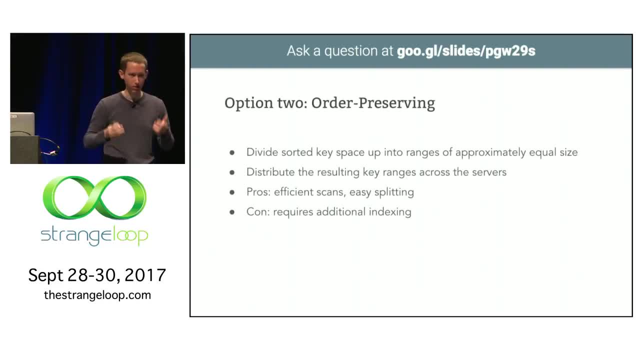 This is really good for range scans, of course, Because we're keeping the data in order. All the data between A and B is in one place. You might have to talk to multiple nodes if you're scanning over a very large range, but 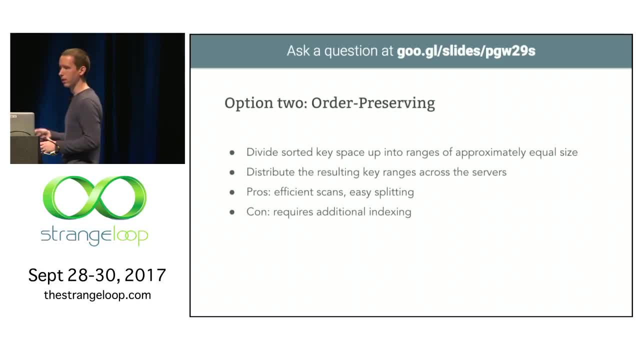 the data is all going to be all in order for you. The downside of this, though, is that you no longer have this deterministic function from a given key to where that key is located, So you have to add on some kind of range indexing structure on top of your actual data to track. 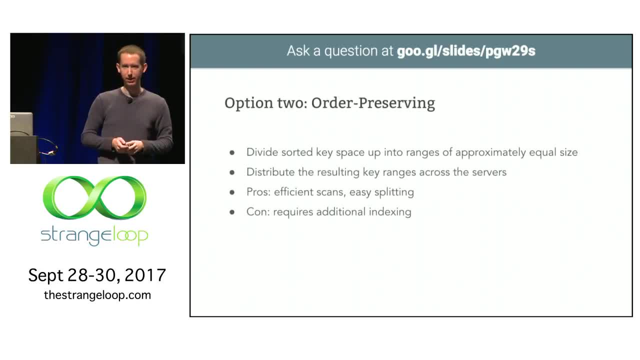 which ranges exist in the cluster and where they're located at any given time. So what that looks like in practice is that you're going to be able to do a bunch of different things. You divide your data up into what we're going to call ranges of data. 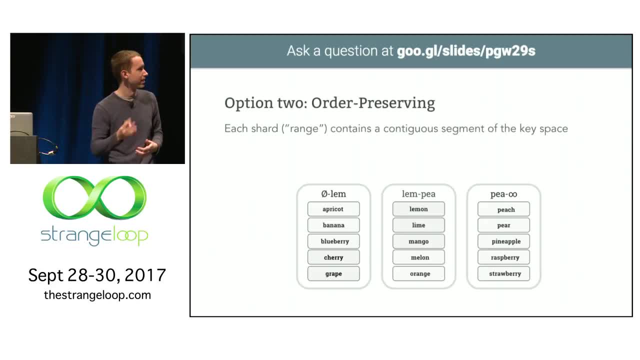 So you have a range from the beginning of the key space through lemon, from lemon through peach and so on, that each just holds the keys and values that fall into that range of data. You also add on this range index on top, as I mentioned. 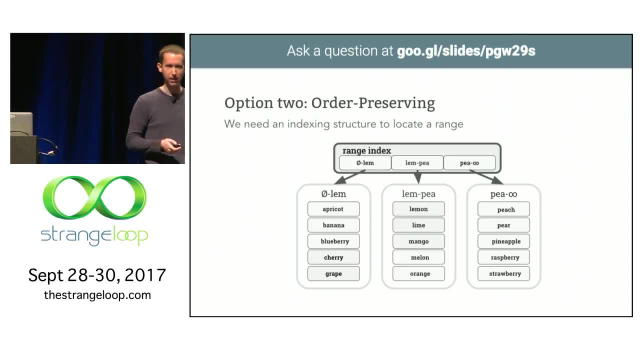 And that's just going to track which ranges exist and where they're located. So any time a query comes in, say you want to read the key mango, you go up to the top of the range index and ask: which range does mango fit in? 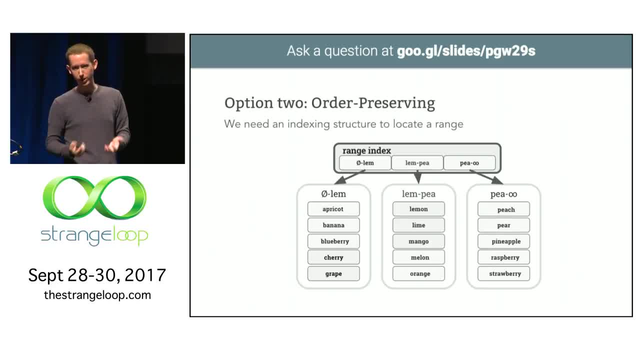 In this case it's going to be the middle one, and that range index will tell you which machines that middle range is located on. So you can then just go send a request to that machine for that key. And it might seem like this is going to add a lot of overhead to all your requests, but 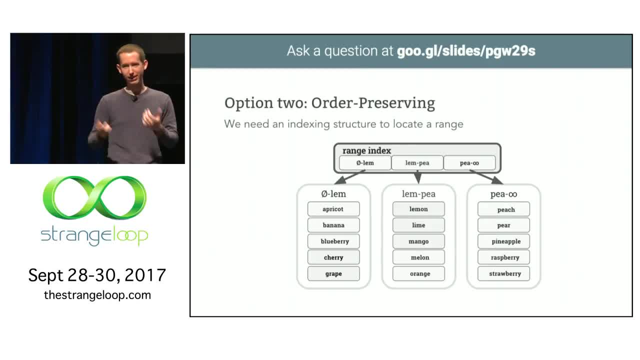 in practice. these ranges don't move often or don't change often, so they can be really easily cached on all the machines. so you don't have to do this extra lookup most of the time And finally, you can do a range scan very easily as well, as I mentioned, 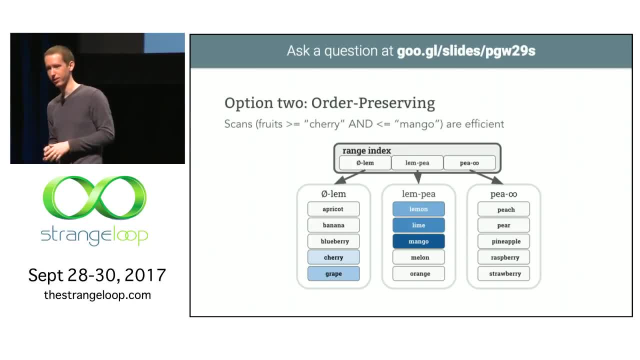 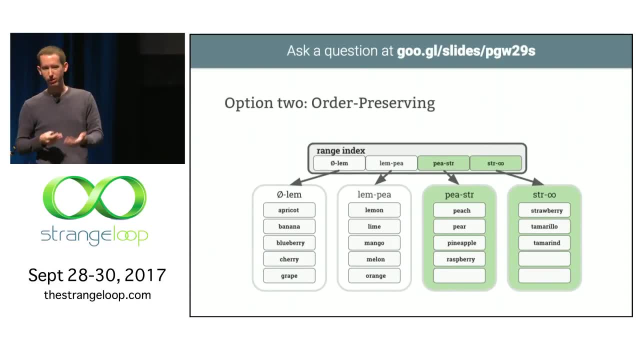 You just look up where the start key is, you look up where the end key is, and read all the ranges that contain any of the data between those points. The last thing you have to ask about this approach, though, is: when do you split up? 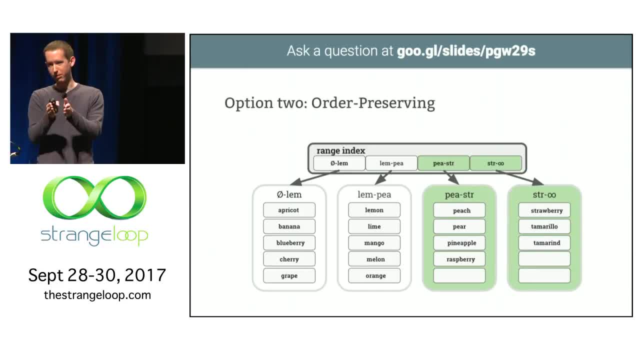 the data, Because you can do a split pretty easily, right, by just picking a point in the middle of an existing range and dividing it in two. So you can divide up that last range, you know, from P to the end of the alphabet, and split it into two if you get a few more keys added. But you have to decide when to do this, So you could wait until the data got too big to fit on a single machine, or maybe you'd do it sooner. In practice, most databases do this when it gets to be about 64 megabytes or 128 megabytes. 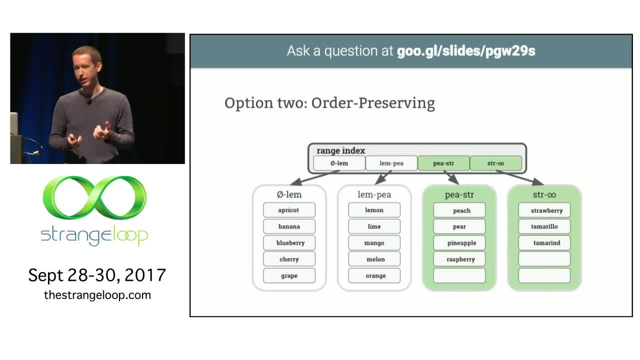 somewhere on the order of 100.. And there's a tradeoff here, because if you let your ranges get too big, then moving them between machines is quite slow. So if you need to quickly move them to recover data from a node that crashed or to rebalance, 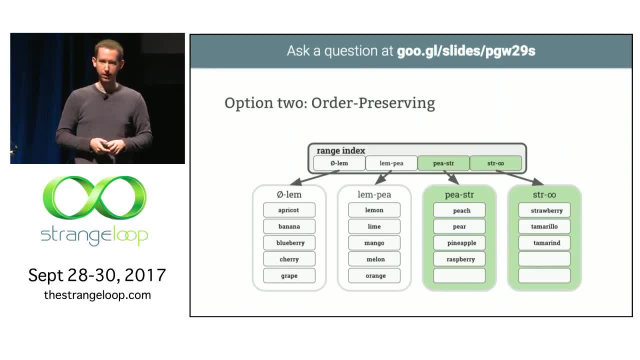 how much data is on each machine. it's tough to do that with ranges that are really big, But if you make your ranges really small then your range index at the top gets to be huge. Having millions or billions of these ranges adds an overhead into the indexing and the 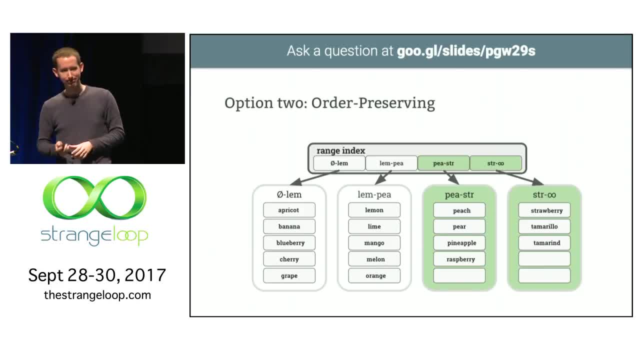 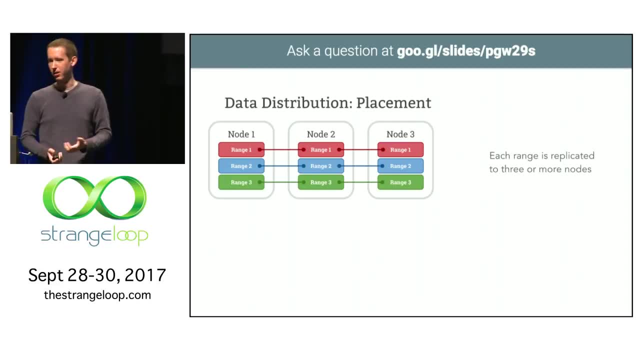 caching of that index, And so you don't want to have tons of them either. And because this is a distributed system, you have to assume that failures are going to happen from time to time. So you might have, or you have to have, multiple copies of your data, such that, if any given 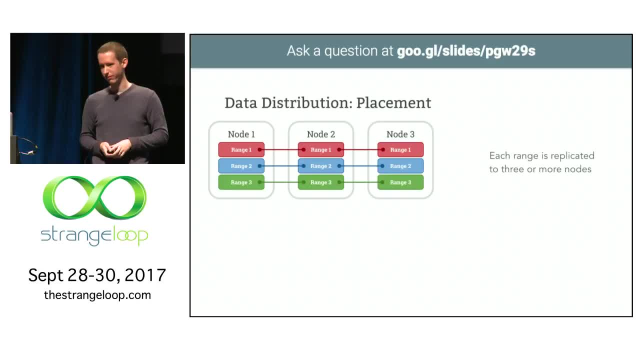 one is on a machine that fails. you'll still have other copies of it available somewhere, And so usually this will be some number, that's three or greater might be user configurable. You're going to spread these around the nodes in your cluster. 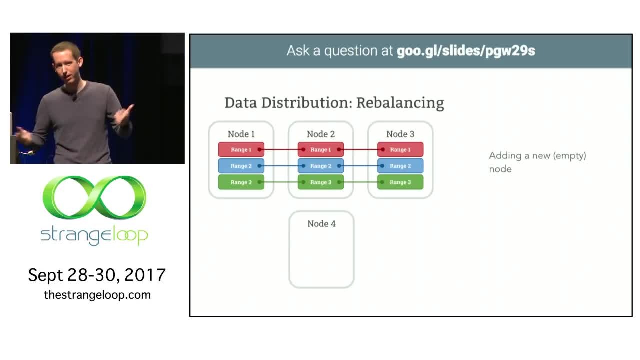 And you have to have some kind of control process that's doing rebalancing. Because what if a new node comes up into your cluster? You know An administrator adds a new machine to your data center. You don't want it to just be empty. 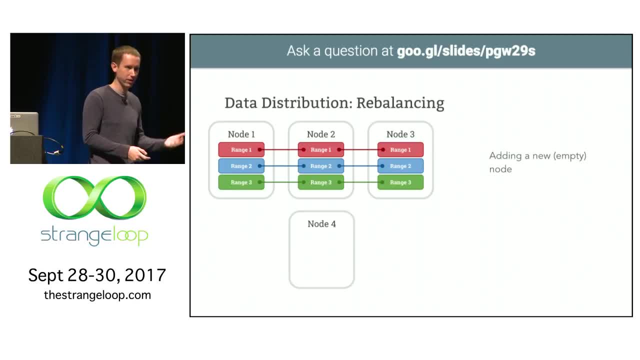 You know you have to proactively move data onto it, And so this control system could live outside the cluster. it could live inside the database software itself. It doesn't make a huge difference other than in terms of how you operate it, But it needs to detect when there's this imbalance of data. 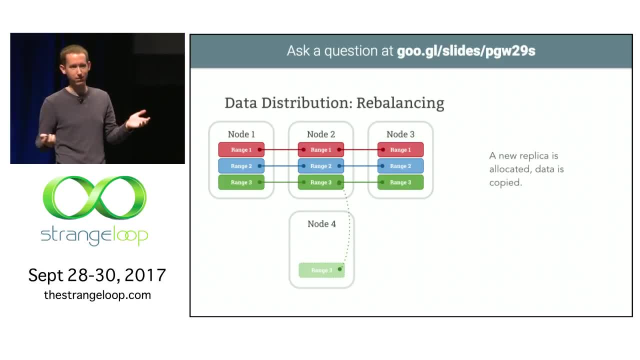 So here nodes one through three have way more data than node four does. So it makes sense to move some copies of ranges over onto node four. So you'll move the copy of range three over there and node three can just wipe that off. 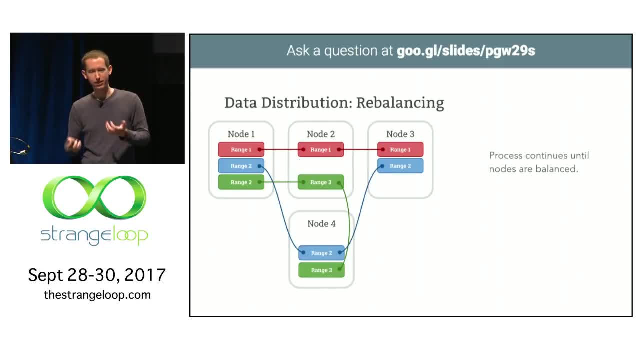 its disk. It doesn't have it anymore. So you can keep doing this until the cluster gets approximately balanced, And you can do this both for the size of the data, the number of ranges in the cluster or even the amount of load. 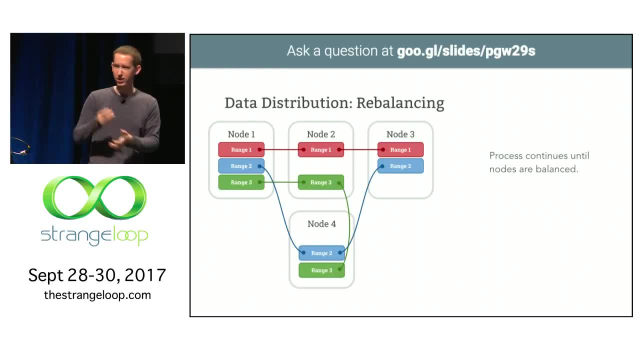 So if some ranges are hotter than others and receive way more QPS, you could split them up into two and spread those out onto different machines in order to balance the QPS on each machine in your cluster, which can be important in practice. There's also the opposite case you have to deal with. 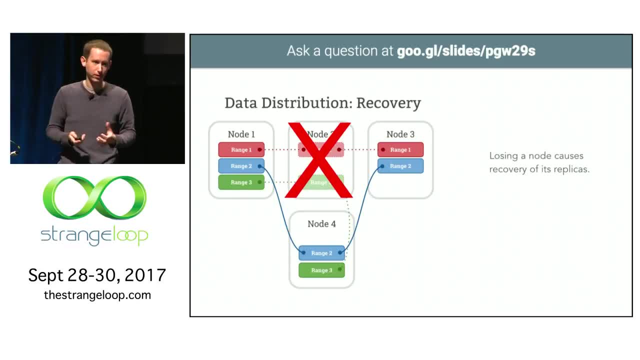 So if a machine fails, you're running with fewer copies of data than you want, Right? So you can replicate these things, create new copies of them so that you get back to the desired amount of replicas at all times, whenever possible. So if node two fails here, we need to make a new copy of both of the ranges that it had. 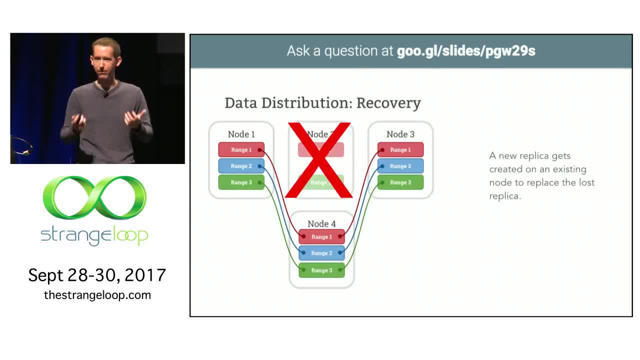 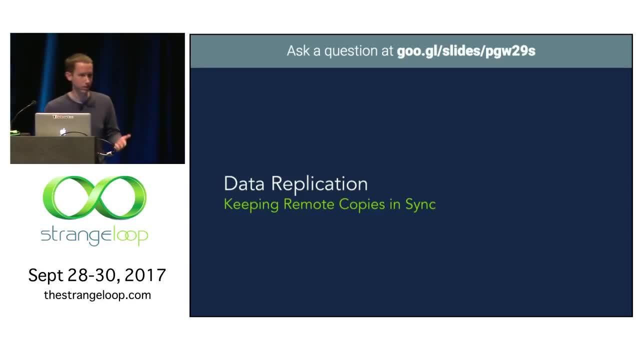 on it And then, if the node never comes back, we'll still be okay and have enough copies. So that's how data gets distributed around these clusters, both in NoSQL systems and in these new distributed SQL systems. But once you do that, as soon as you have multiple copies of data in a distributed system, 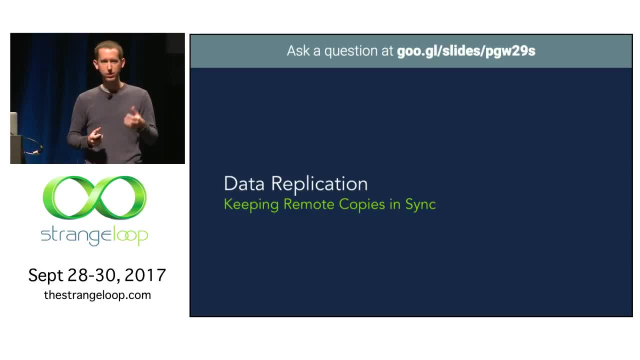 you really need to ask yourself: How are you keeping them in sync? Or how are you dealing with conflicts where one copy says one thing and one copy says another thing? Because it's bound to happen: Network requests will be lost, A machine will be down and might not be up to date. 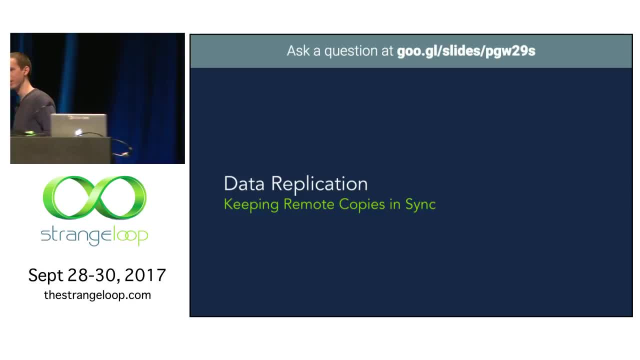 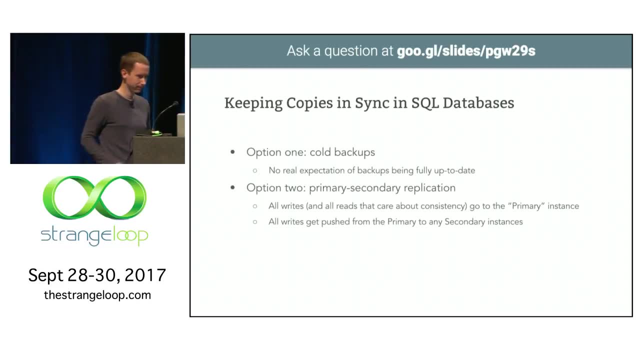 And you need to have some way of deciding which copy is correct at any given time, And so SQL databases, since they store all their data on one machine, don't really have to deal with this, unless they're running some form of primary, secondary replication. 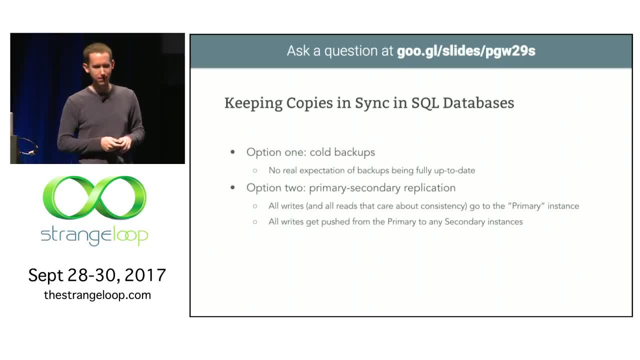 So that's one of the things that we need to be careful about. We need to be careful. If you're running primary secondary replication, there might be an expectation that your secondaries are up to date, Because the way primary secondary replication works is just that you have one copy of your 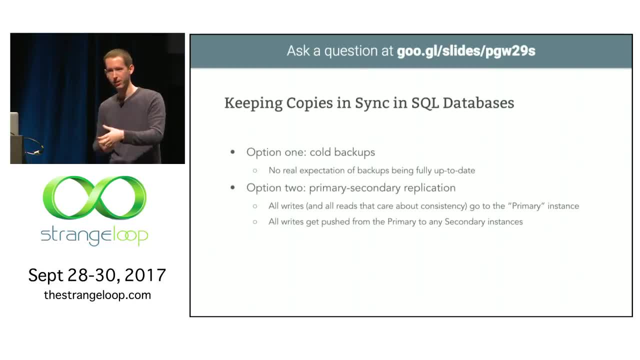 database that's considered the primary, where you send all of your writes and oftentimes all of your reads, And the primary will just take each write, write it to its own disk and then at some point send those writes off to the secondaries so that they can have the same copies of the. 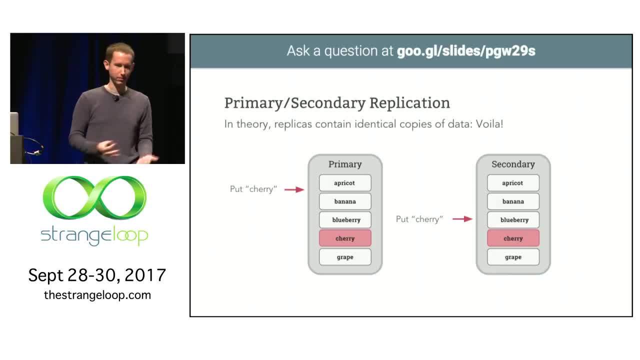 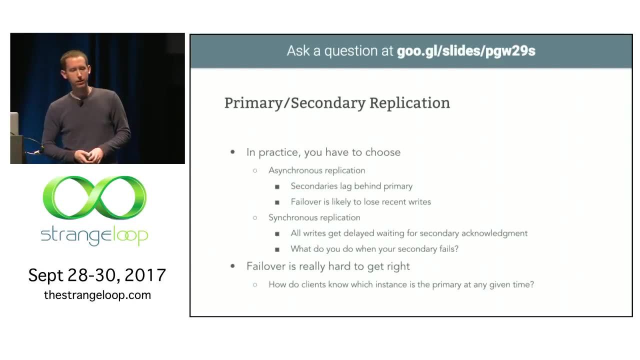 data And in theory it's a very simple concept, right, The primary gets a write, it writes it to its disk and it passes it along to the secondary or the multiple secondaries. In practice, there is a bit more complication. 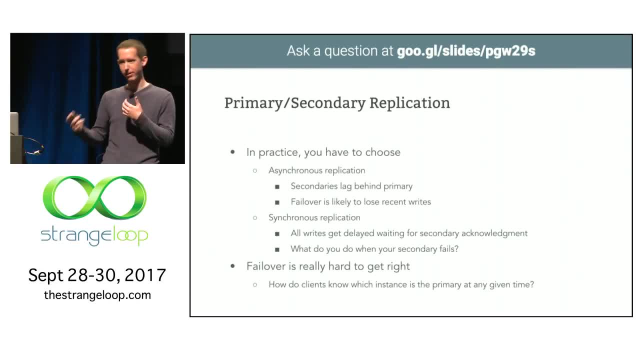 There are edge cases where you're going to lose data or where you're going to be reading stale data, And it's tough to really manage this. as an operator, You have to choose between asynchronous or synchronous replication, where asynchronous just means the primary will write a write to disk and acknowledge it to the client. And in the background it will start sending those writes off to secondaries. What that means is that the secondaries won't necessarily have all the data the primary has. If you have to do a failover, you could be losing recent writes. 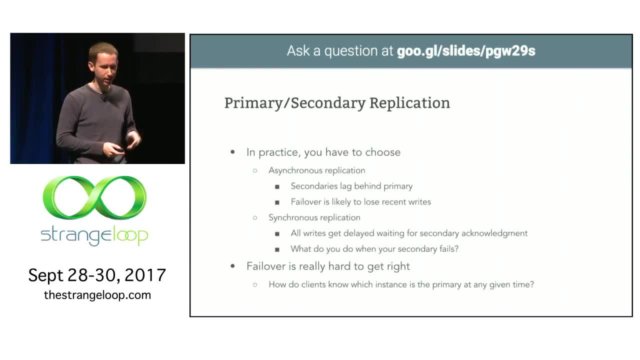 If you're doing reads on the secondary, you could be missing out on recent writes. If you do the opposite approach- what could be called synchronous replication- that would mean that you're waiting on the secondaries to write the data to disk before telling clients. 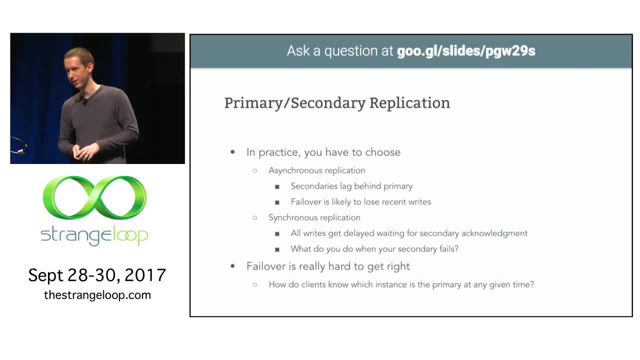 that their writes have succeeded. This is going to introduce extra network delay into all of your write requests and it also introduces interesting questions Like what if the secondary fails, or what if the secondary gets slow? How long are you willing to wait on that secondary to respond to a request before you just give? 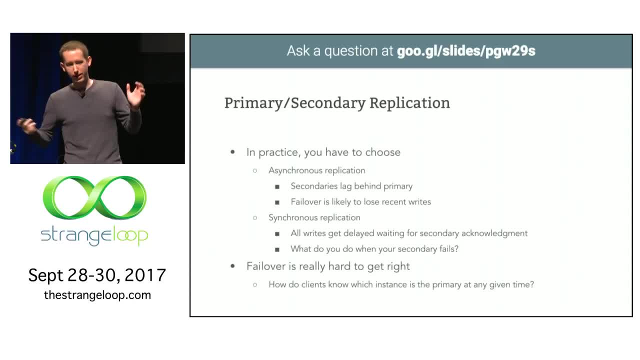 up on it. And either way you do this failover is really tough to get right because you have a lot of clients in your data center presumably talking to this database and they need to know which one to talk to at any given time. 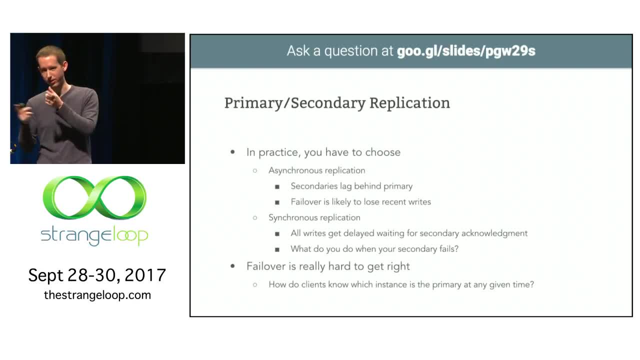 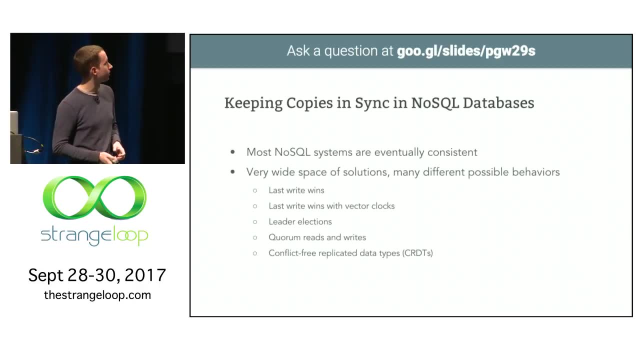 So it's tough to fail them all over without some straggling requests potentially going to the wrong instance and leading to a sort of split brain. All right, Moving on to NoSQL. NoSQL systems really do a whole ton of different things to keep track. 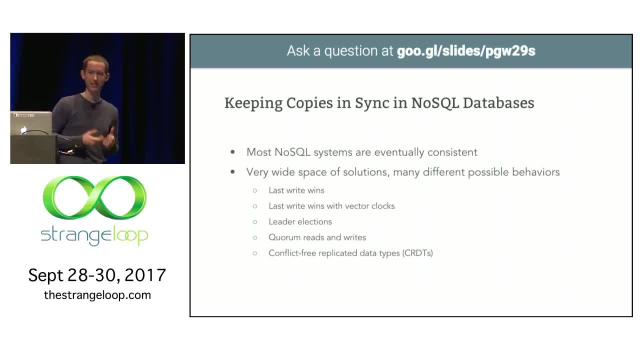 of their copies of data, And most of them are what's known as eventually consistent, which is kind of just a euphemism for not consistent. Most of these different solutions for maintaining copies of data can fail in weird ways, whether there are partitions or not. 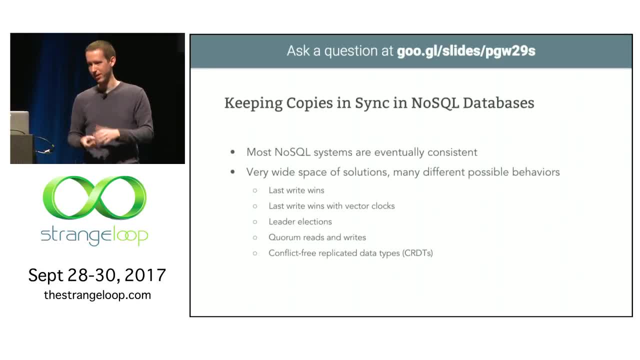 They could be dropping writes. if two writes come in for the same keys around the same time, One of them is just going to clobber the other And it's nondeterministic- They could be serving up stale reads. So if you do a read in an opportune time, you might be getting an old piece of data. 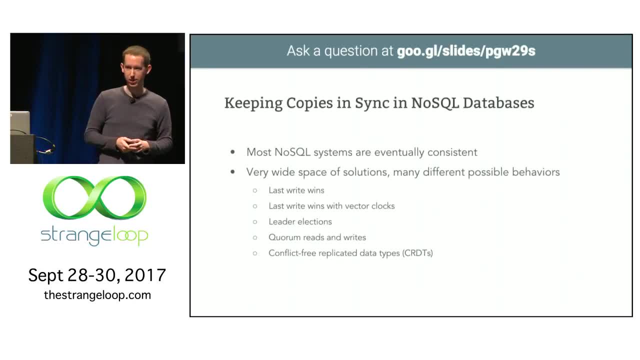 In some situations you might get an uncommitted piece of data, something that was never really acknowledged to be committed. The only solution here that really can be called eventually consistent, in that, if you wait long enough, the data will truly be consistent, with nothing lost, is these conflict-free replicated. 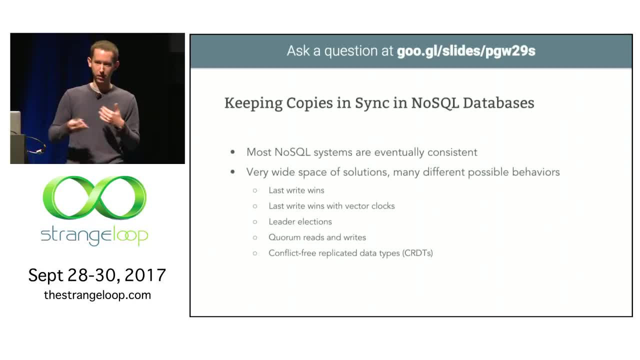 data types. These are some really cool algorithms that have been talked about at past Strange Loops, So I'd recommend checking out those videos if you want to learn a little more. But they do, in fact, keep all your data consistent if you wait long enough, if you let all the 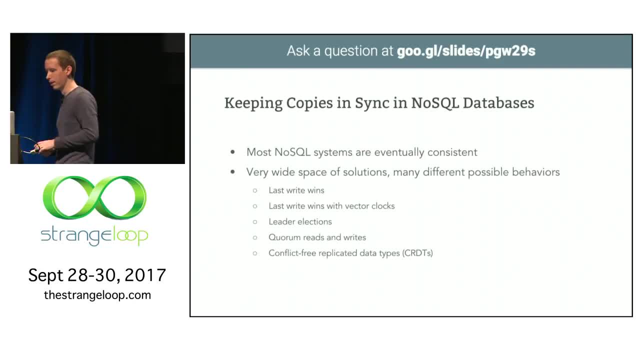 data from the different machines eventually converge. We don't have enough time to really drill into the details of how all these different things work. You could fill multiple really interesting talks just doing surveys of all the different mechanisms NoSQL databases use to keep their data in sync. Just know that typically they really don't keep data consistent in any way. You could lose data, get old data, et cetera. Keeping copies in sync in NoSQL databases usually works in similar ways between all the systems, which is a pretty serious change from NoSQL. 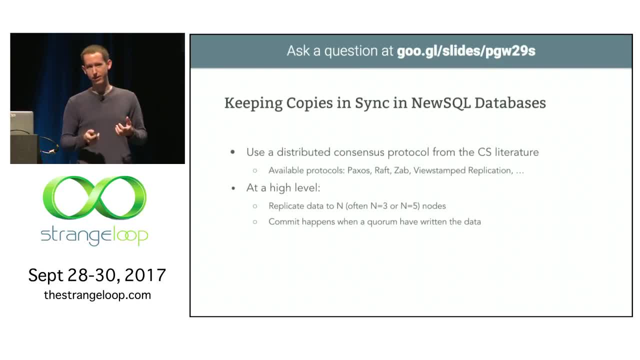 Most NoSQL databases or distributed SQL databases use what's known as a distributed consensus algorithm And these consensus protocols have been very heavily researched. There's a lot of academic papers proposing different ones, proposing improvements and variations on the existing protocols, And they've been proven through formal methods to be correct to keep your data consistent. 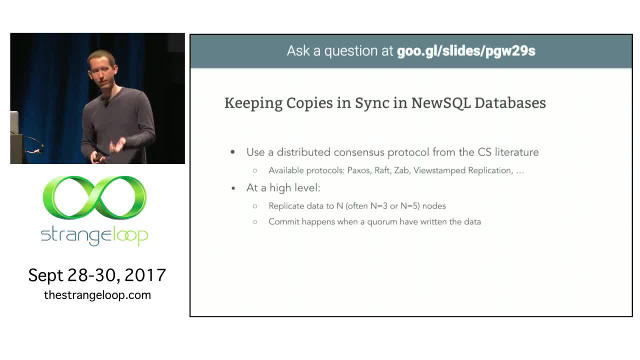 and reach agreement. The most famous of these protocols is Paxos. It was originally written about 30 years ago almost, but is notoriously hard to understand and hard to implement, So there aren't really many implementations of it. Google wrote a paper on how many years it took them to get one of these implementations. 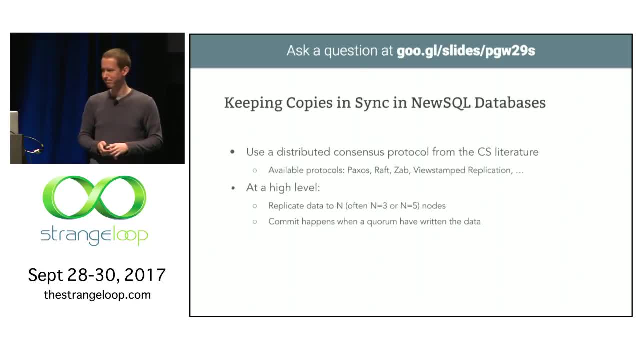 into a usable, reliable, production-ready state. It's really not easy. Raft was a new protocol written about five years ago by a PhD student at Stanford. that has really taken off because it was designed from the get-go to be correct, but much more. 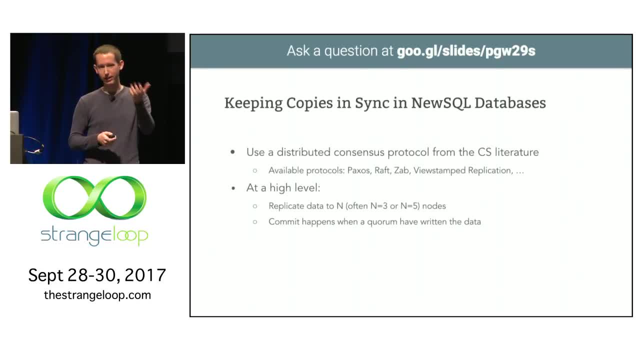 understandable and easier to implement. So now you can go out on GitHub and find open source implementations of Raft, just already written for you, that you can throw into your own system and use to get reliable replication of data. It's not necessarily easy to use, but it's available if you want to use it. 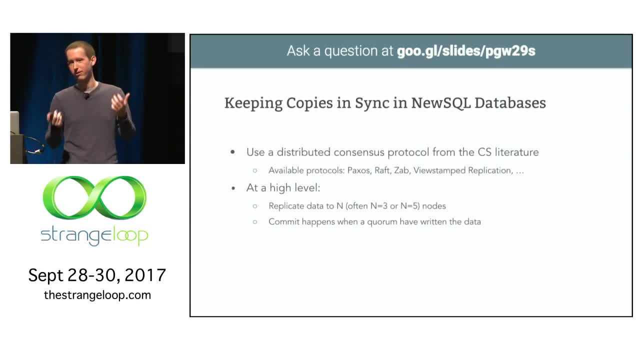 And so this has made consistent systems much more possible, much easier to write than they were 10 or 20 years ago, because these protocols have become simpler, easier to write and more widely available. But the way that these protocols have changed over the years is that they've become much. 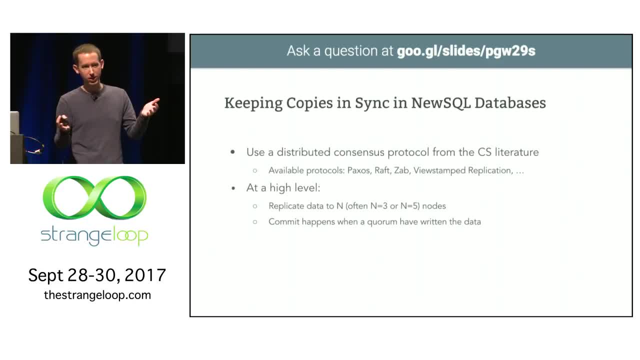 easier to use. The way that these protocols typically work is that they have some odd number of machines in a cluster, so three or five, maybe seven, And commit just happens when a majority of those have written the data to disk. There is more in the details that makes them always correct, but that's the high level. 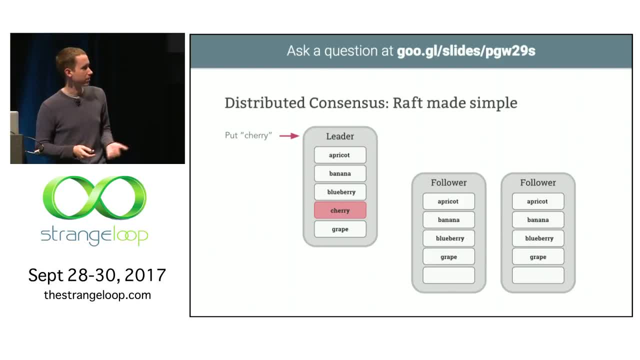 And so let's take a look at Raft in particular. Raft is what we use in CockroachDB. We share an open source implementation with lock, with the lock-oriented database at CD, And it's a pretty hardened implementation at this point. 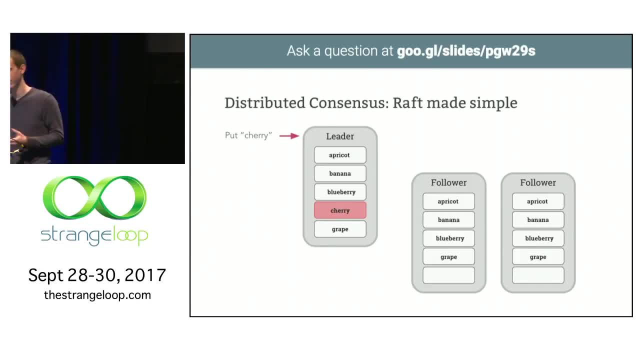 And it's a pretty hard implementation. And Raft is based around leader election. So if you wanted to describe Raft in three sentences, you'd say you have a set of replicas that elect a leader And that leader appends incoming commands to a sequential log and assigns an index to 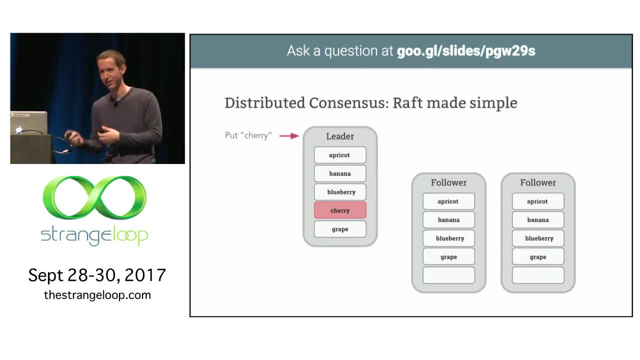 each command And if you've been to past range loops, you've probably seen talks on how sequential logs. are these really powerful constructs in distributed systems? So you have these writes being appended to a sequential log And then that log just gets replicated from the leader to the followers. 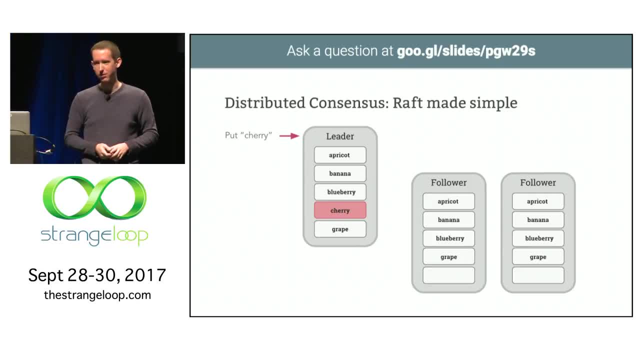 And the commands are considered committed Once a majority of the nodes in the system have written them to disk. So in this example, if a write comes in for the key cherry, the write has to go through the leader, because all proposals in Raft have to go through the current leader. 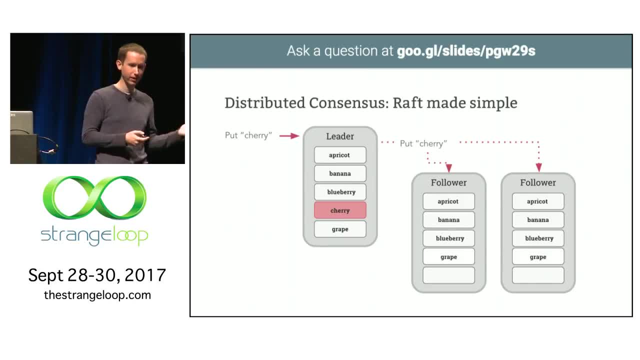 So the leader will write it to its own disk in that sequential log and replicate it to the followers. As soon as either of those followers has written it to disk, we suddenly have it written to disk on a quorum of them, right? So we have two out of three. 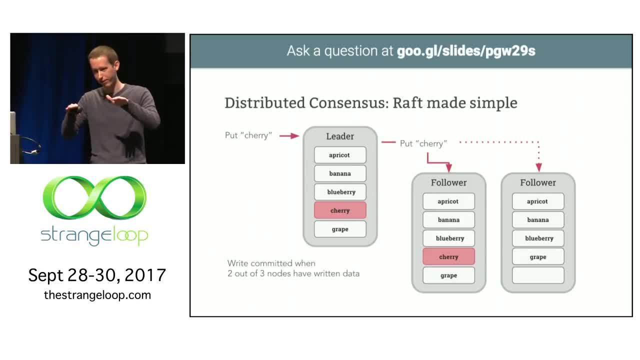 At this point the write is considered committed. even if all the machines were to be suddenly turned off at this point, That write would have been predicted And at this point normally the follower will acknowledge it to the leader and the leader can acknowledge the write to the client. 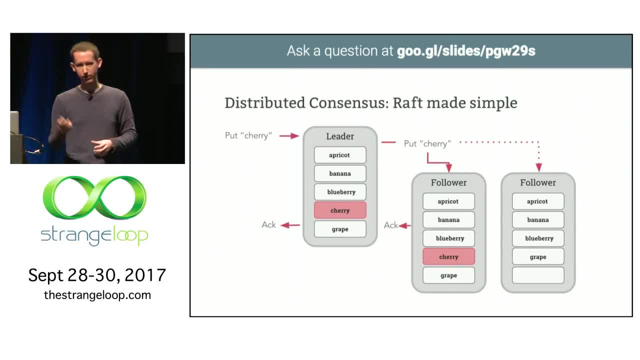 So you do have to wait this one network hop before you can acknowledge writes, which is a bit different from those SQL databases that just have everything in one place. But notice here that you didn't have to wait on that third replica to write it to disk. 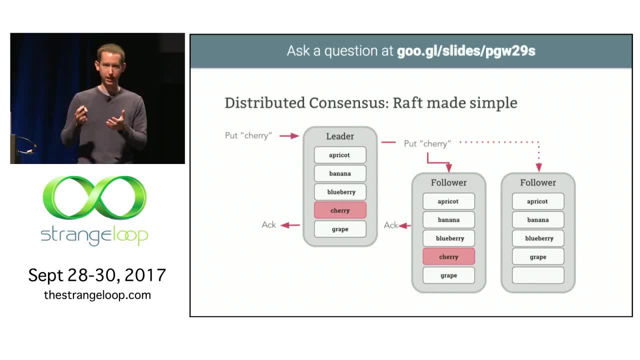 All that these algorithms require typically is a majority to be up to date. So if one node is running slow for some reason, or say it gets shut off for a few minutes, or it's on the other side of the country, You don't have to wait for it, which allows for some interesting configurations where you can deploy two replicas on the east coast and one on the west coast, and those two that are close together can operate and serve these writes really quickly because they don't need to wait for the one that's far away. But that's what happens when things go well. 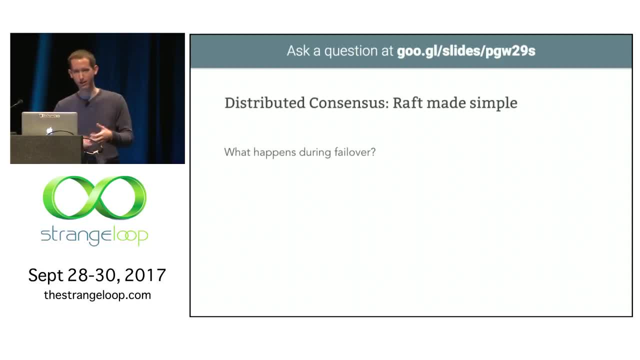 And, of course, you need to ask yourself what happens when things don't go quite so well. That's always a question in distributed systems, because you're going to have failures, you're going to have partitions, you're going to have all sorts of problems. 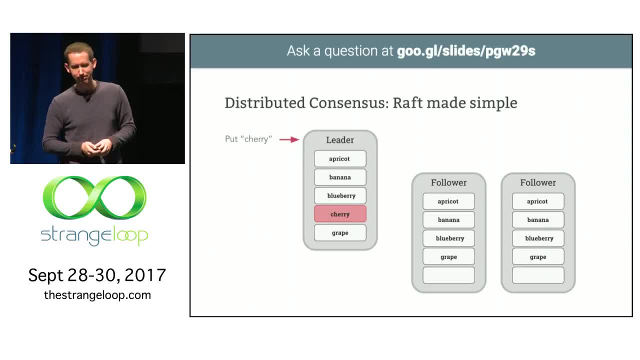 And so if we have the same example where a write comes in for the key cherry And the leader dies before it's able to replicate it, By the definitions we've been given, that write has not been committed because it's only on one hard drive, right? 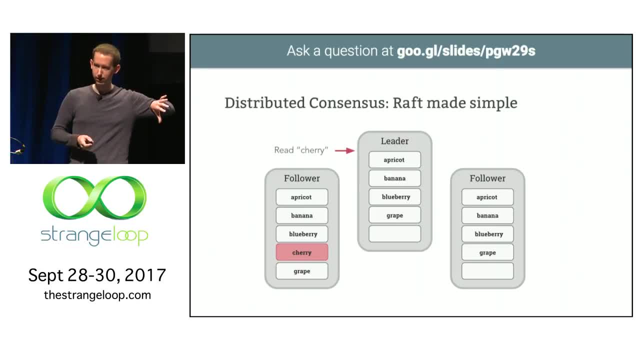 So those two followers are going to elect a new leader while that old one is down. So we have the new leader. now the second replica has become the leader and it doesn't have that key because the two replicas that were followers didn't know about it. 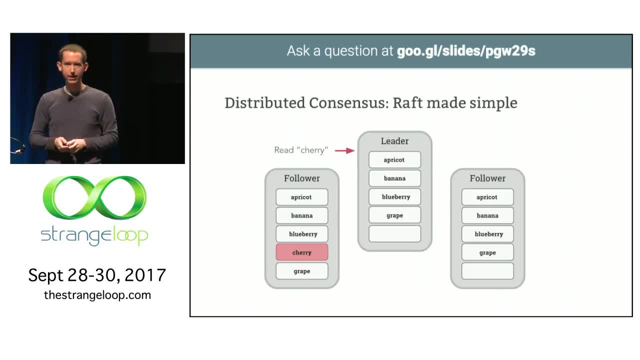 So they didn't know that the leader is supposed to have this key. So Farid then comes in for that same key. According to Raft, according to the consensus protocol, that key was never written. It's only on one disk and the leader doesn't have it. 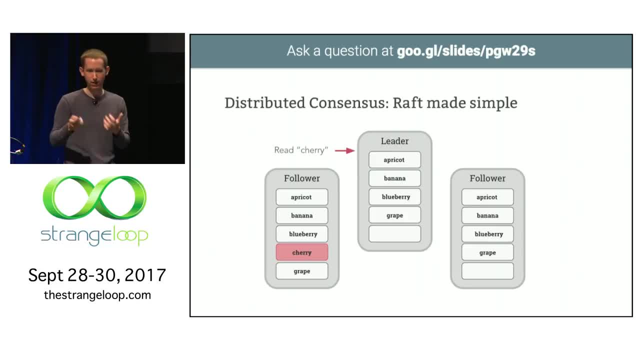 So the leader is going to go to its followers and say, hey, do you have this key? No, no, I don't. The first replica will then have to be asked to remove it because it was never truly committed. And on a leader changeover, any uncommitted proposals just get dropped. 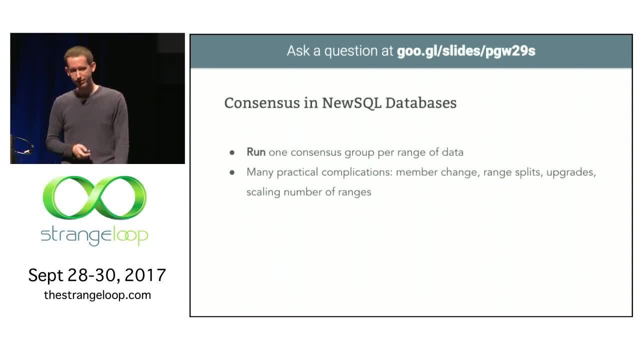 And so at this point, the key is just returned as not found, And that's like a surprisingly thorough overview of Raft. I mean, there are more details, of course, But it is a very- It's a very understandable algorithm. I'd recommend reading the paper if you're interested in this kind of stuff. In practice, new SQL databases like Cockroach and Spanner have to run one of these consensus groups for each range of data. So in that example from earlier we had those three ranges and three or four nodes. 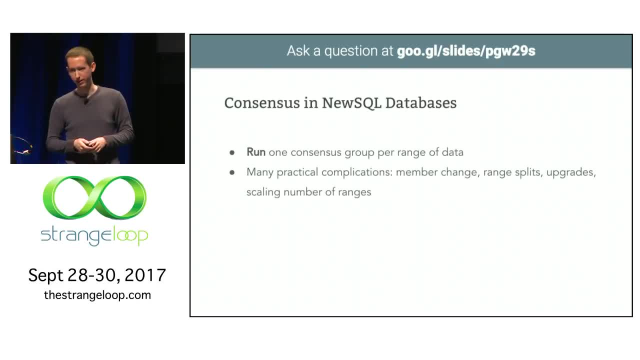 We'd have to have one group for each of those ranges. so three consensus protocols running in the cluster And in practice we have way more than three ranges. right, because we're restricting them to be about 64 megabytes. So if you have terabytes of data in your system, you could have hundreds of thousands of these. 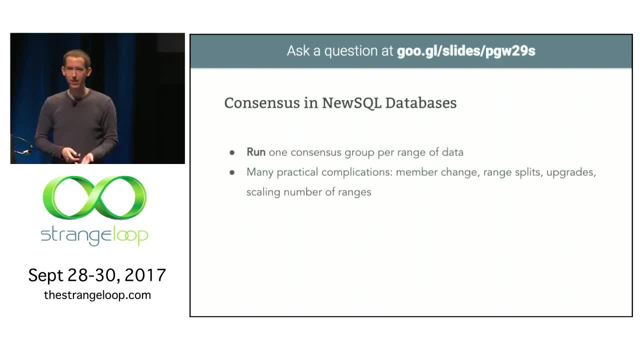 ranges. So there are a lot of engineering complications that come into play in these systems. It's tough to scale, to have this many ranges and to be able to handle member changes when you're moving them between nodes, to handle, splitting them consistently to deal with. 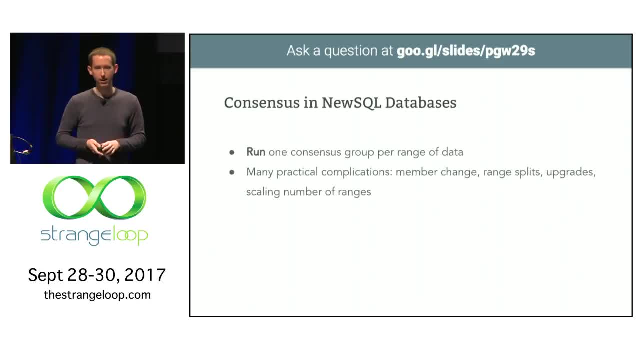 software upgrades, where some nodes are running different versions of the software than others. But these are all engineering complications that can be dealt with through just hard, diligent work, assuming you have the solid foundation of research underneath you telling you that this replication is correct. 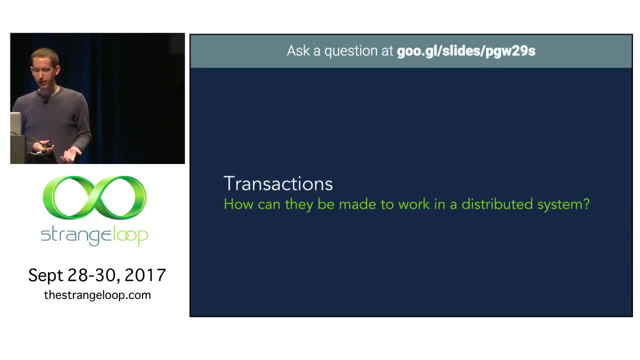 And so, finally, let's take a look at transactions. So we have consistently replicated data on a per-range basis, But SQL databases allow transactions to touch any rows anywhere in the system. So you have to handle coordination between these ranges, between these consensus groups. 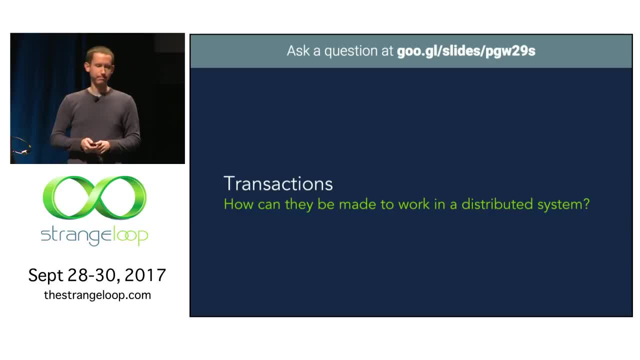 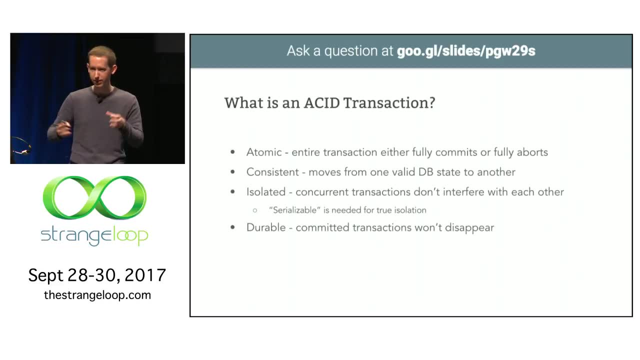 And so these groups might be on different machines all throughout the cluster. And when we're talking about transactions, we're talking about good old, old-school ACID transactions, Where you can have any combination of reads and writes that touch any of the data in your 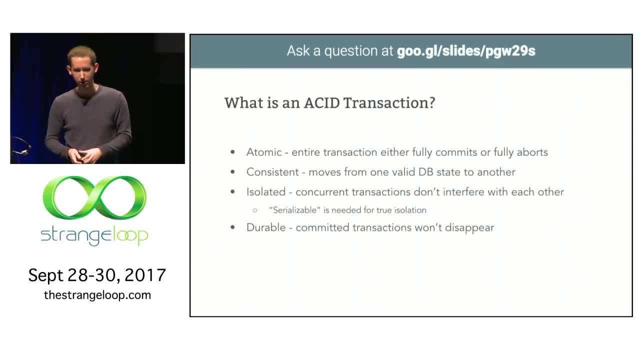 system that are atomic, consistent, isolated and durable. The two more interesting facets here, the two tougher ones to provide, are being atomic and being isolated. Consistency is really just about checking user-defined constraints like uniqueness constraints or foreign key relations and things like that. 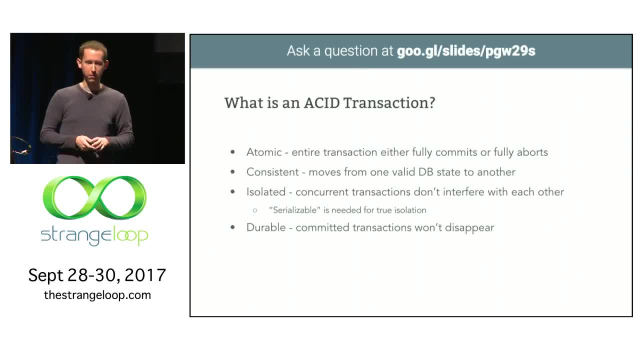 And durability is really just about synchronizing your rights to disk properly, But the hard parts, from an architecture perspective, are being atomic and being isolated. Let's take a look. And so atomic means that all of the rights that are sent together as part of the same. 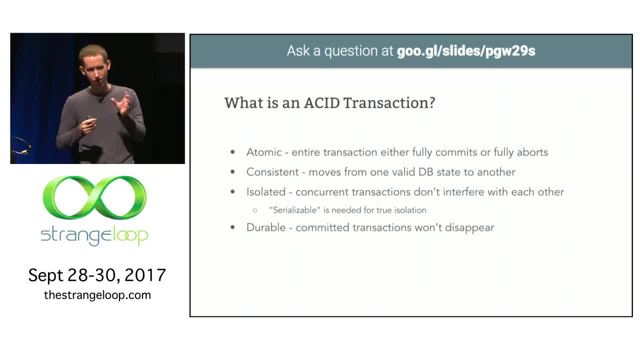 transaction either commit or none of them commit, You have to get all or nothing. And being isolated means that having concurrent transactions trying to operate on the same data in the system that they can't interfere with each other, So it's as if they all have their own correct, consistent view of the database at all times. 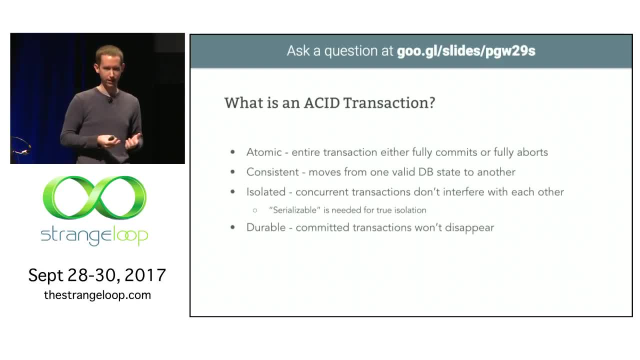 And there are multiple isolation levels, but we're just going to focus on serializability today, because that's the isolation level at which you don't get any anomalies, you don't get any incorrect data back out of your database And the serializable level is required by the SQL standard to be truly compliant. 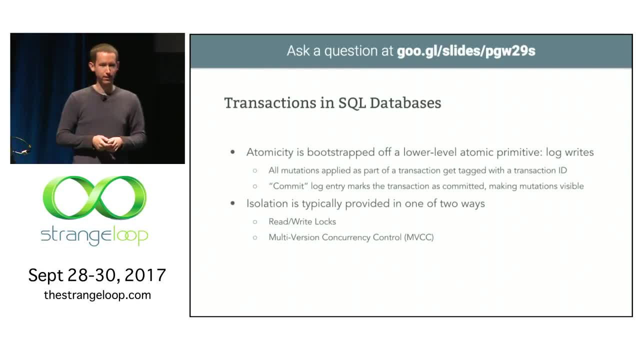 So first let's look at SQL databases, And a lot of SQL databases are proprietary, so I'm focusing specifically on Postgres here. The way that Postgres does atomicity is that all the mutations that are applied as part of a transaction, all of those rights, when they get written to disk, they're written. 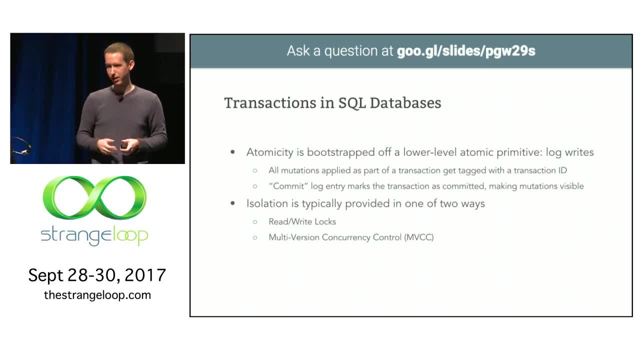 with the transaction ID associated with them or attached to them. So if I write to the key cherry, it's going to have this little marker next to it saying it was written as part of transaction foo. And those rights aren't considered to be visible to reads, necessarily, because they're still. 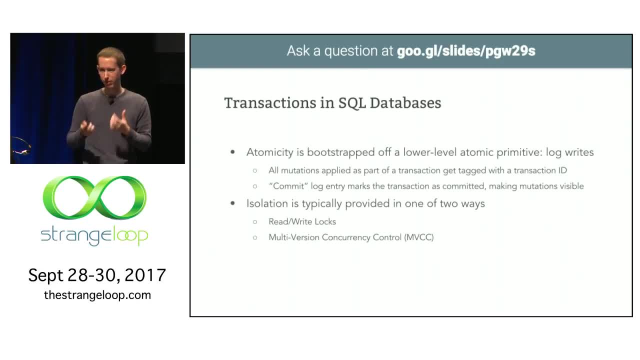 tagged with that marker, And transactions have to know which transactions have committed or not. When you do want to go ahead and commit the transaction, you have to write it to this commit log. And that's where the atomicity comes in, because you can do a single write to a disk block. 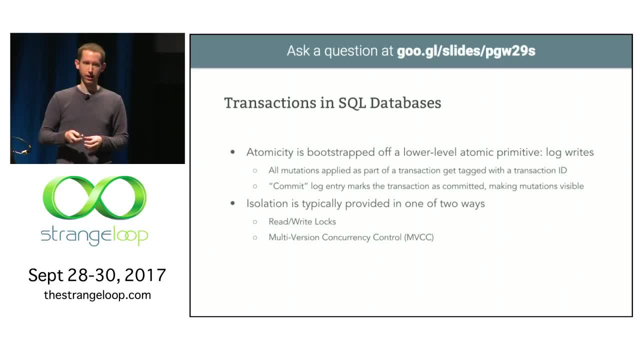 in an atomic way, And so if we can do this single disk write to the commit log to mark that transaction is completed, then we have in one fell swoop committed every operation that happened as part of the transaction, And that one disk write will either fully succeed or fully fail. 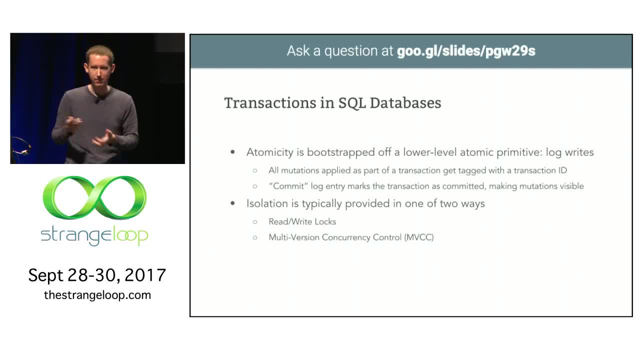 That's guaranteed by the disk. So that's how you get atomicity of all these writes spread out over the entire system to be committed all at once. You boil them down to just this one disk. write Isolation is provided in a couple different ways, which we'll look at individually. 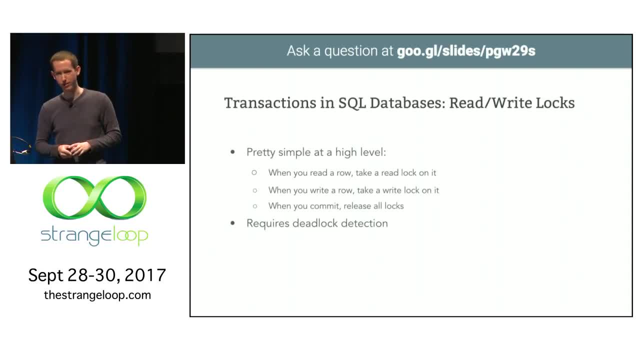 Read- write locks are the easiest way, or the simplest way, to provide isolation between transactions. This is how SQL databases did it for decades after their creation, And it's exactly what you would think. It's the same as using a read- write mutex in your own program. When you want to access a row, you take a read lock on it. When you want to write a row, instead of read it, you have to take a write lock on it And read and write. locks exclude each other right, because that's how read write mutexes. 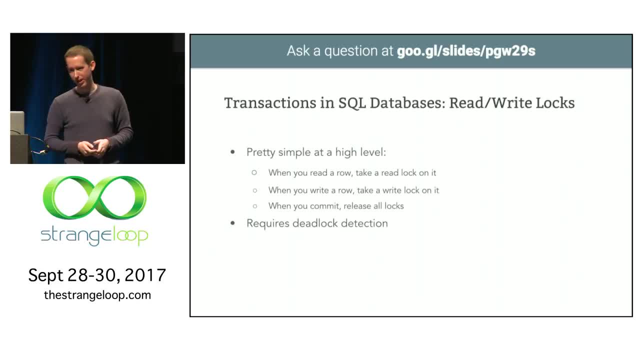 work And then you have to hold these locks until you commit and release the locks once you've committed your transaction. So the database has to do some deadlock detection. But this is pretty simple to understand And pretty simple to implement as well. There are ways to reduce your isolation level by releasing locks earlier on in the transaction. 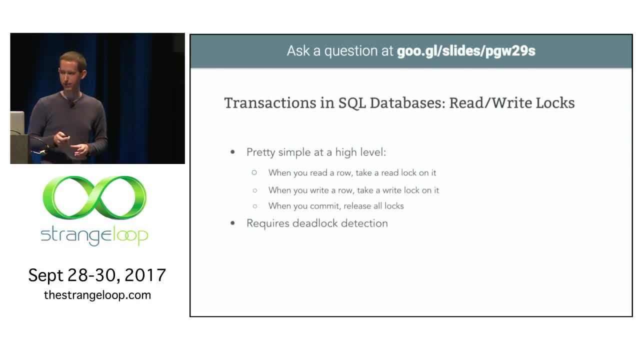 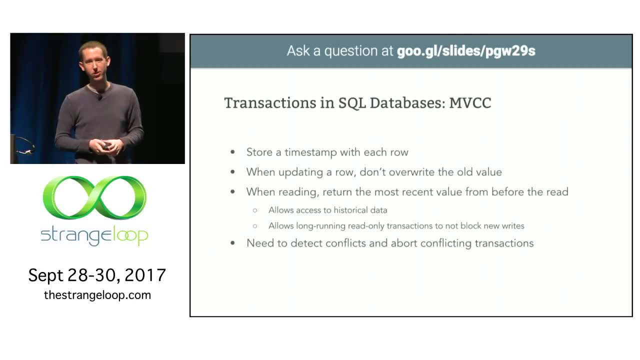 But then you'll have potential anomalies appearing in the behavior the user sees. The other approach to doing isolation in SQL databases is what's known as multiversion concurrency control, or MVCC for short, because that's quite a mouthful- And what this is is that any time you write a row to disk, you store a time stamp along. 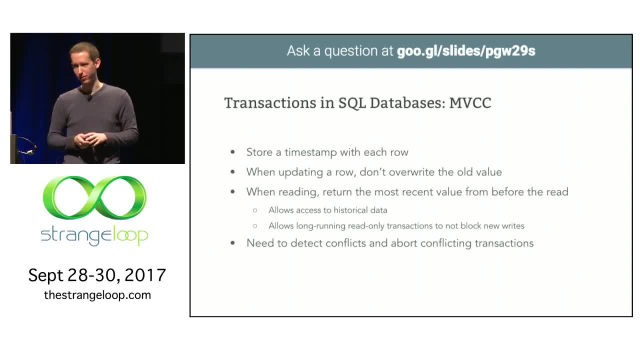 with it And that time stamp represents the time stamp. And any time you update the row, rather than overwriting the row on disk, you have to just write a new row next to the old one with a new time stamp. so you're not getting rid. 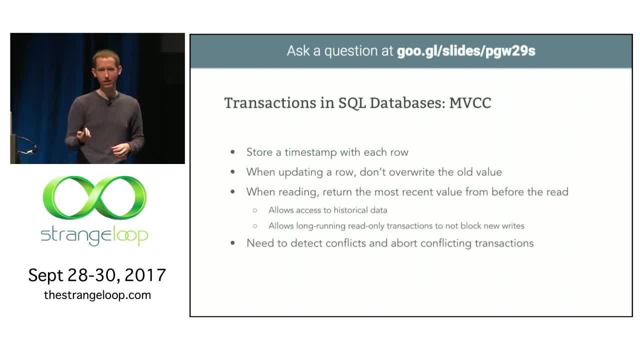 of the old data, And then anyone that wants to read a particular row has to get the most recently written version of that row from before the read zone time stamp. This has a few nice properties and it allows access to historical data because we're not. 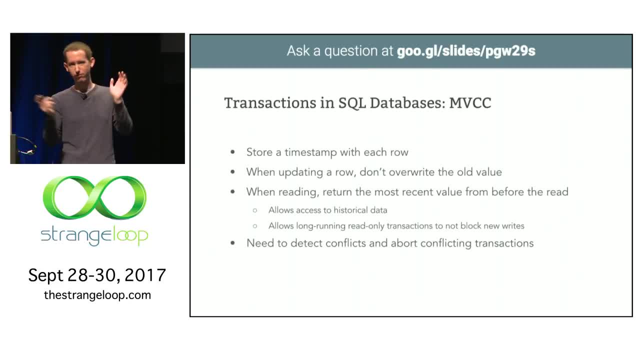 deleting and overwriting the rows. you can run a query as of 24 hours ago and get a consistent view of what the state of your system was then. This could help you track down things like bugs in your application that have started writing funny data to your database. 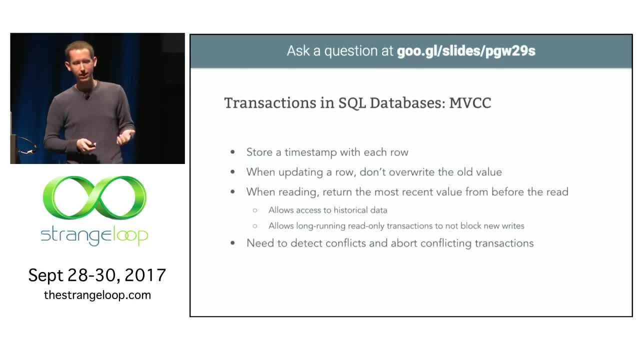 You can pin down when the issue started happening. And the other big win is that it allows long-running read queries to not exclude other transactional workloads from happening, because you're not holding onto these write locks anymore, You're just running at an older time stamp and not blocking anything else from happening. 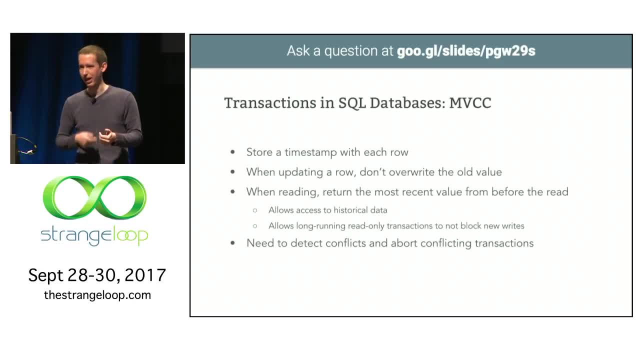 So MVCC by itself doesn't really provide isolation. You have to have conflict detection on top of this In order to do that. you have to have a conflict detection on top of this. In order to do that, you have to have a conflict detection on top of this. 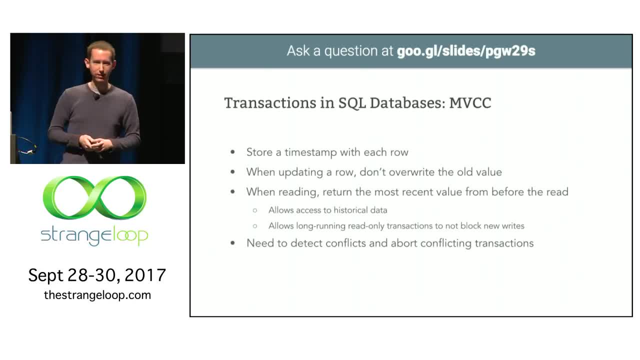 In order to do that, you have to have a conflict detection on top of this, So you have to be able to tell when a transaction is trying to write or read to a key that something else has also been accessing recently, So it's a little tougher to implement. 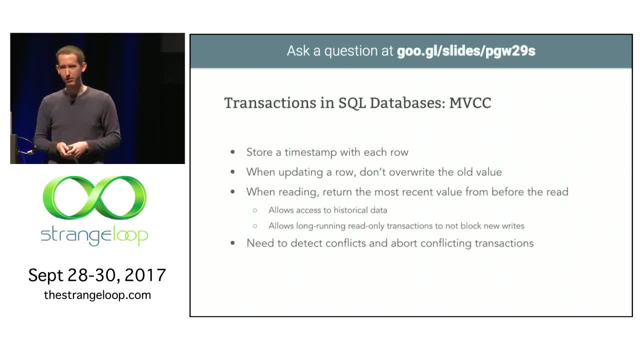 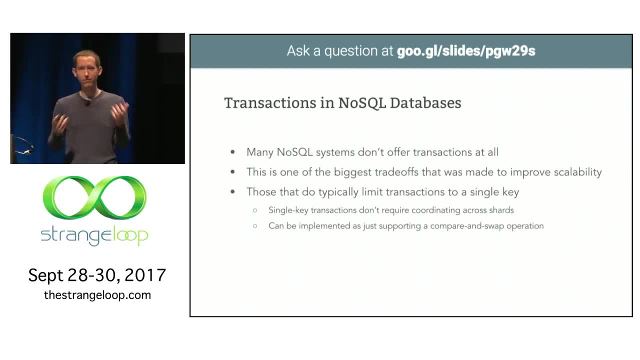 Postgres implemented a version of this, I think about a decade ago, that it uses for certain isolation levels now, And so NoSQL systems don't have a whole lot to talk about because they, just as a rule, don't really offer transactions. The best thing you're going to get in most NoSQL systems is a single key transaction. 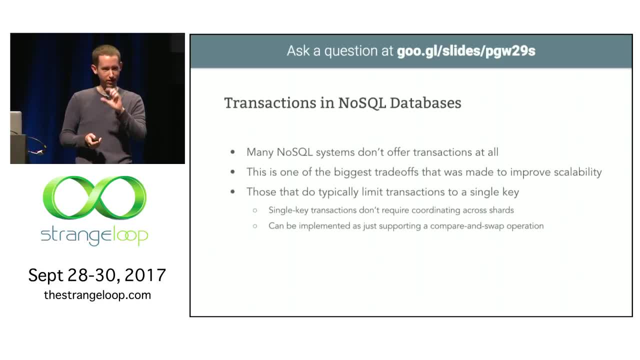 So you might be able to do a read, modify, write loop on just a single key, but you won't be able to atomically commit multiple keys at the same time. or, you know, write some keys on one part of the system, then do some reads, then write some keys somewhere else. and have that all happen as an atomic event. It's just something that they sacrificed in order to achieve scalability at the time, Because transactions imply coordination and coordination is hard in distributed systems, So it was going to be a lot of engineering work for them to try to do this. 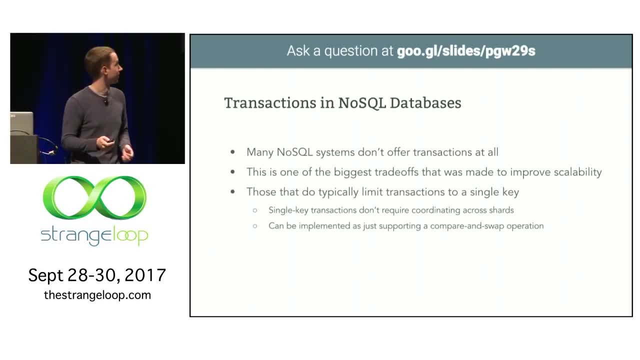 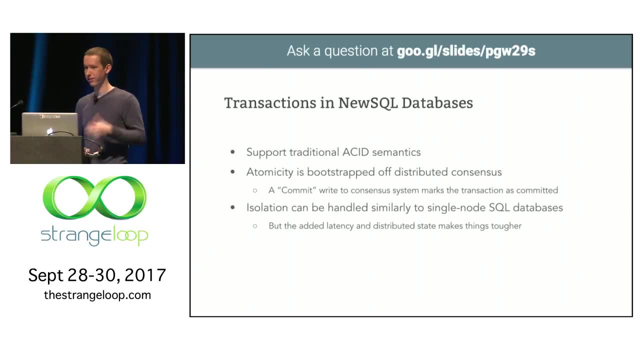 And so you know. this is kind of all I can really say about NoSQL transactions. Finally, distributed SQL has to support the same semantics as traditional SQL databases, because you can't replace a SQL database as a drop-in replacement unless you have the 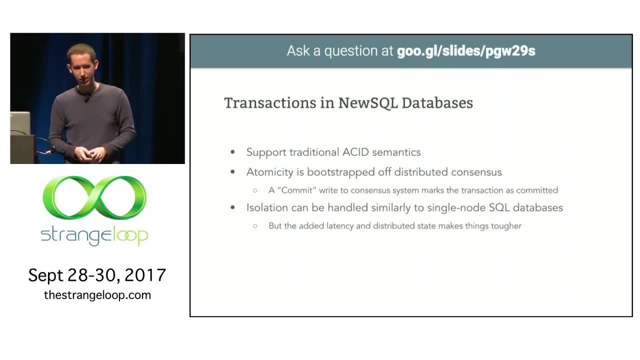 same semantics. So we need full ACID, we need serializable isolation, and that takes a bit of work in a distributed system. But we can learn a lot from how SQL databases do it, So we can provide atomicity in a similar way. 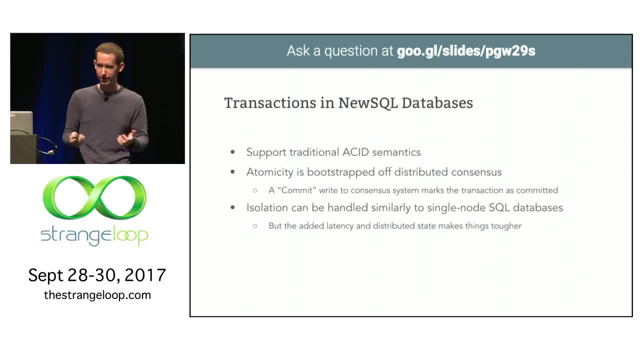 All right, All rights that come in as part of a transaction can be tagged with a transaction ID, as usual, And we just have to have this transaction record somewhere in a consensus group, Because rights to a consensus group, a Raft group or a Paxos group are atomic. 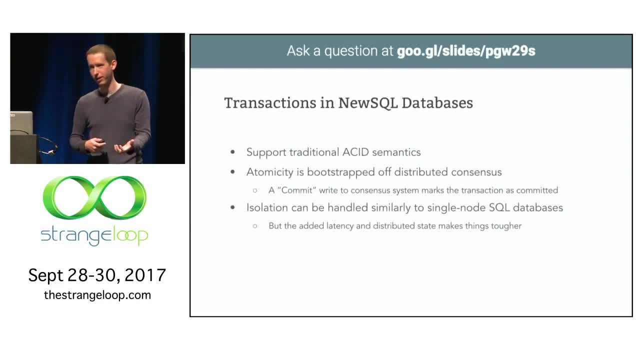 They either do happen or they don't. So whereas a single-node SQL database can use a single disk right to get atomicity, we can use a single consensus group right. So it just takes that flipping of the transaction status from in progress to committed to mark. 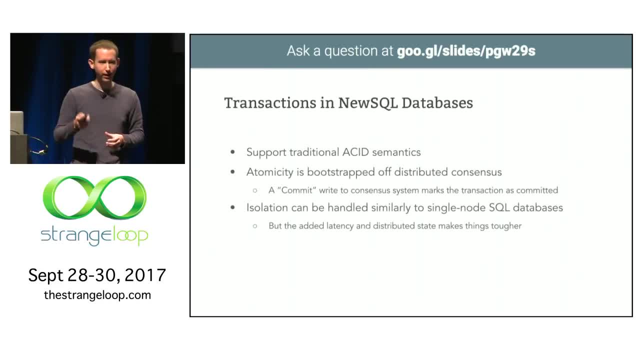 it as done and to mark all of the rights involved as done. And isolation can also be done somewhat similarly to single-node databases. It's a bit harder due to the network latency involved and the fact that all the state isn't being held on one machine in the same memory space. 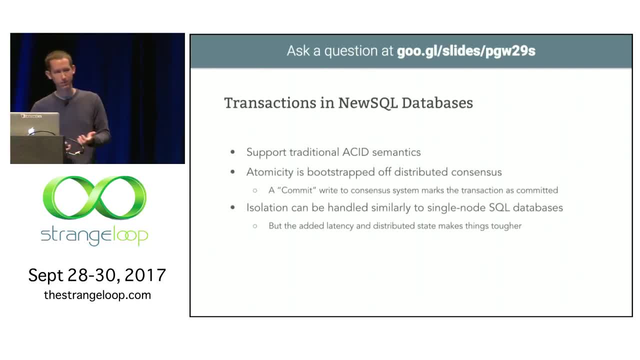 But we can use similar approaches. I think most new SQL systems that I'm aware of at least use some form of MVCC. Spanner uses a combination of MVCC with two-phase commit and two-phase locking. They have to rely a lot on their very special hardware clocks that are in the Google data. 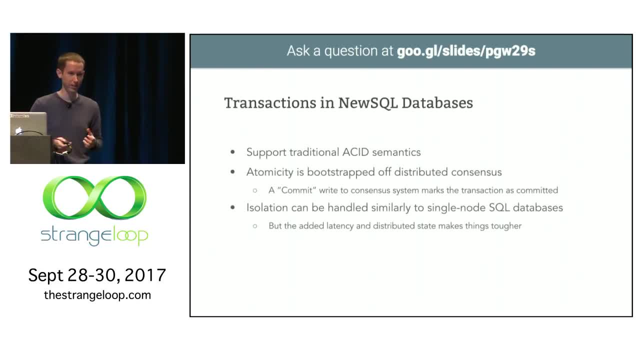 centers. these days, CockroachDB uses pure MVCC with conflict detection and it has to use a combination of hardware and software clocks to make this work reliably over widely distributed networks. So if you do have replicas on both coasts of the US, for example, 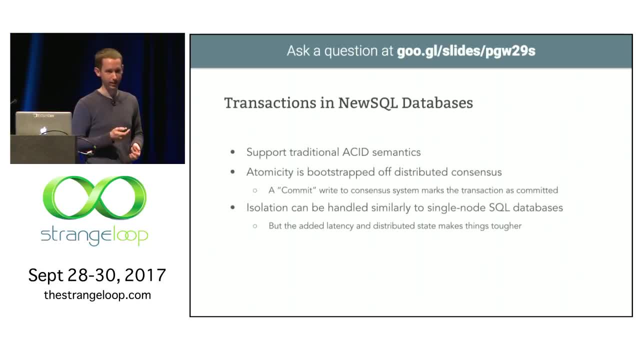 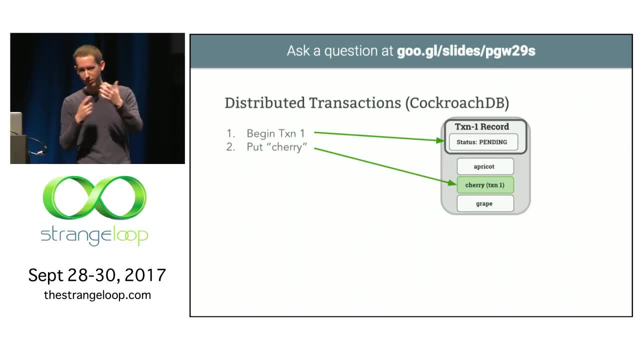 But let's take a look at this MVCC and conflict detection approach to transactions. So you'll start by beginning a transaction and putting a key to the database And that key will be in some range And, for convenience, In Cockroach at least, we put the record for that transaction, tracking its status in. 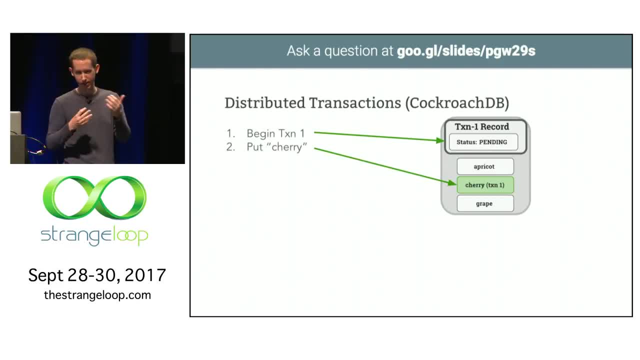 the same range as that first write so that they're co-located if the entire transaction happens to be happening in just that one range. So you'll start the transaction and you'll write the key And notice that the key is tagged with the transaction number which we're just using. 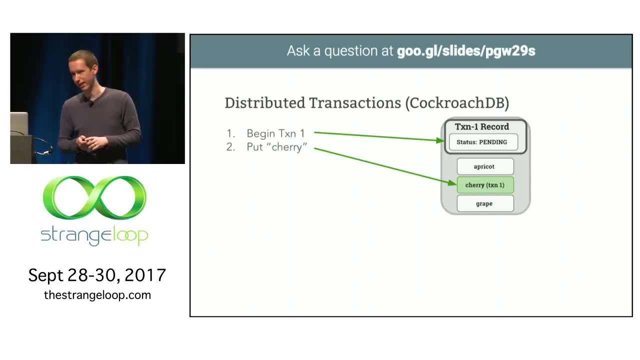 one in this case, And that's to indicate that it might not be committed yet. If some other transaction comes along and wants to read the key cherry, it's going to have to check the transaction status for that transaction to be aware of whether or not it. 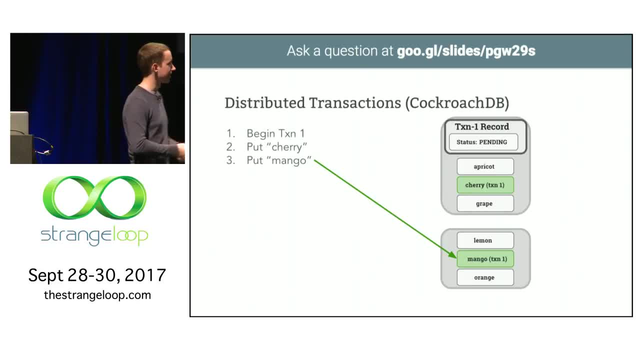 should be returning that key. The transaction can go off and write keys in other ranges of the system, other tables of the SQL system and so on, So it could write mango in another range And then, when it's done, it just has to go and do a single consensus write to flip the. 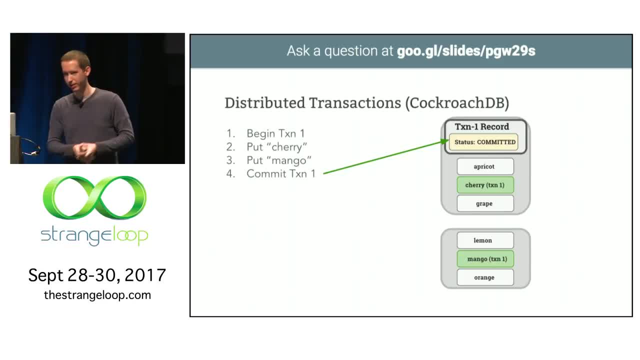 status of the transaction record. So it's going to mark it as being committed And at this point the transaction is done. Any new transaction that comes along and reads those keys will know to just go check the status of the transaction and it will see that it's committed. 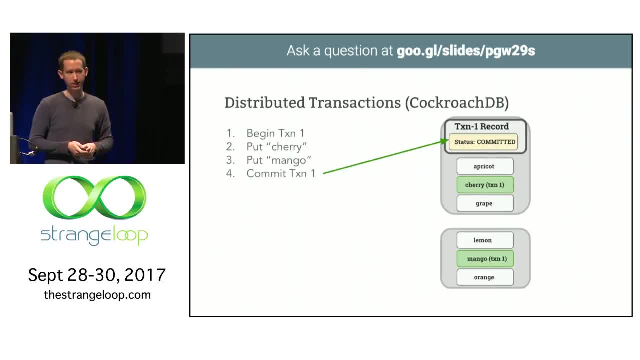 That does add some extra work to the reads, though, And so after a transaction finishes, it goes and proactively cleans up those transaction ID pointers, so that anything that comes along later to do a read doesn't have to go do that lookup, And once we've cleaned up the pointers we can also just get rid of the transaction record. 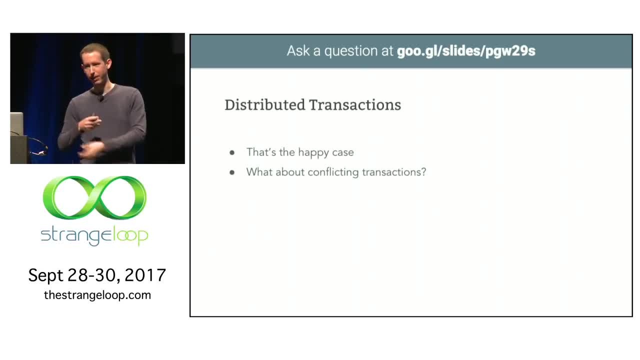 because it's not needed anymore. But again, any time you're talking about one of these distributed systems, you have to ask about what happens when things fail or when things conflict, when things don't go wrong in general. So let's take a look at one particular type of conflict. 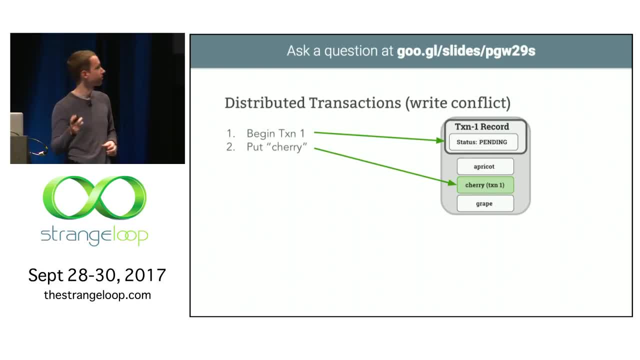 It's going to be a write conflict, So the transaction will start out in the same way. It will write a key and put a transaction record for that transaction into the same range, But then another transaction is going to come along and try to write to the same key. 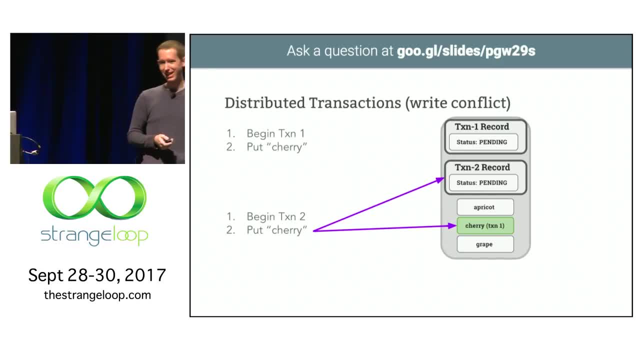 And so in this case the state to detect that a conflict has happened is on the range itself. So the machine that's currently responsible for serving queries for that range knows that something else has written to that key recently. So we have a conflict here, but we've also detected it. 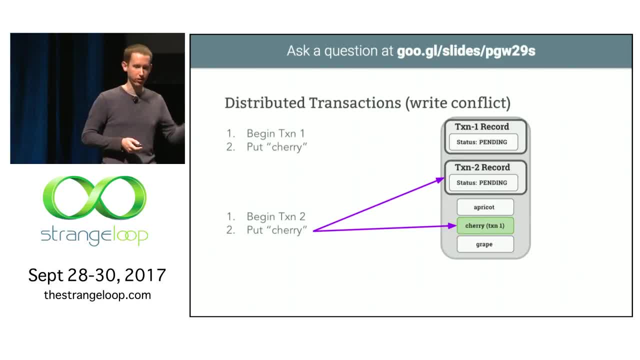 Okay, There are multiple ways to try to handle this. You can make the transaction wait on the first one that's already running, or you could do an abort of one of the two transactions and force them to restart, And so, assuming we're going with the abort method, you have to pick one of the two to 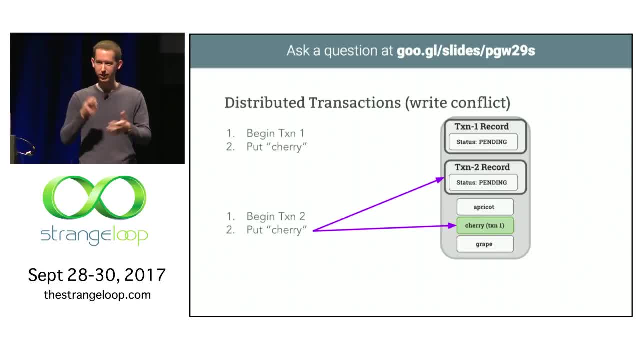 abort, And so this can be done with a priority scheme, so transactions can have a priority assigned to them when they start. It could be user assigned, it can be randomly generated and you make the higher priority transaction win, for example, so it's less likely to be aborted by a lower priority one. 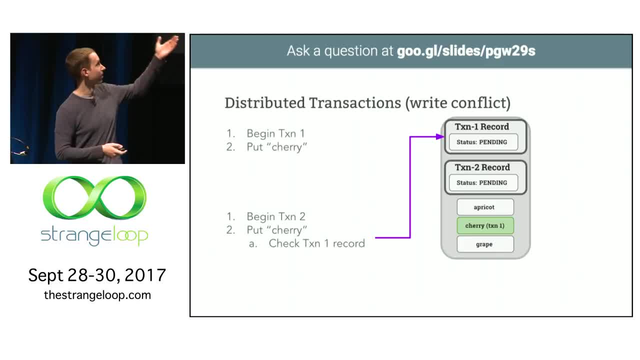 Okay, Transaction two, you know, has to check whether the transaction one is done, though, because maybe transaction one is already done and transaction two doesn't have to worry about it. In this case it's not, though, So transaction two is going to decide to push or abort transaction one. 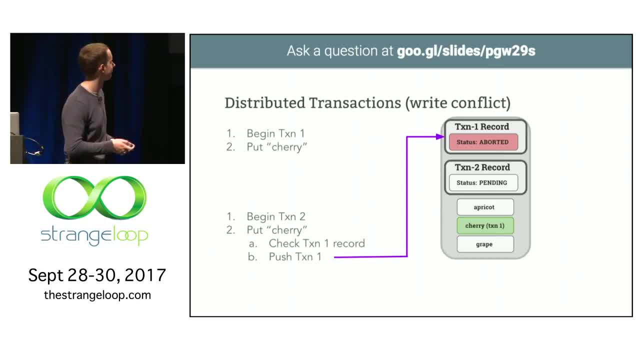 Push would just mean to make it have to start over at a higher time stamp. So transaction two has aborted the conflicting transaction. It can update the write to its own key, where intent just means the transaction ID tagged on it, And then commit. 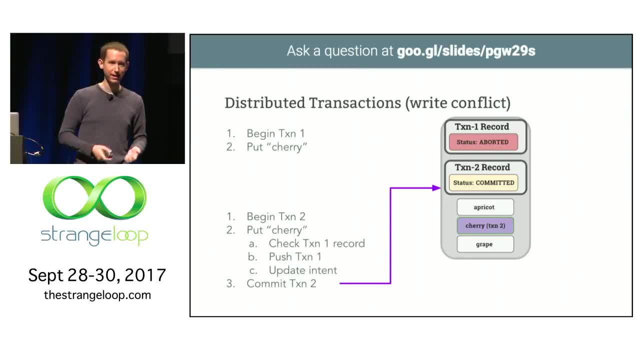 Okay, Transaction two is done and transaction one is going to have to restart. It might be able to do this restart internally to the database or it might have to send that abort message, the abort error, out to the client for the client to retry. 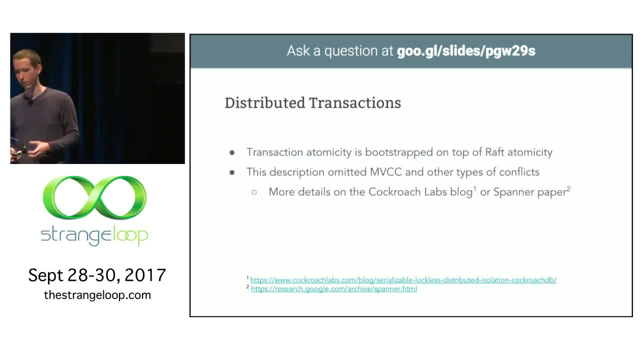 So that's a quick overview of how these conflicts work, of how these systems work. More details can be found on the Cockroach Labs blog in the Spanner academic papers- other descriptions of these systems online, because this description had to omit things. 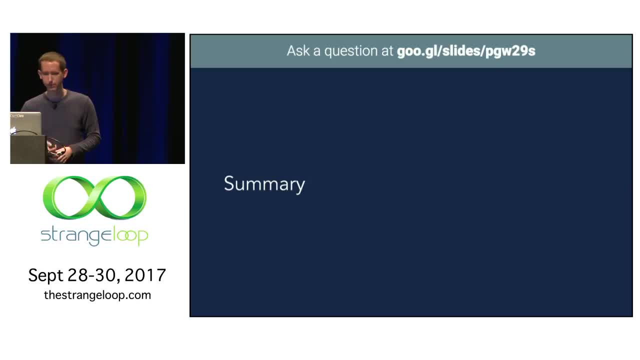 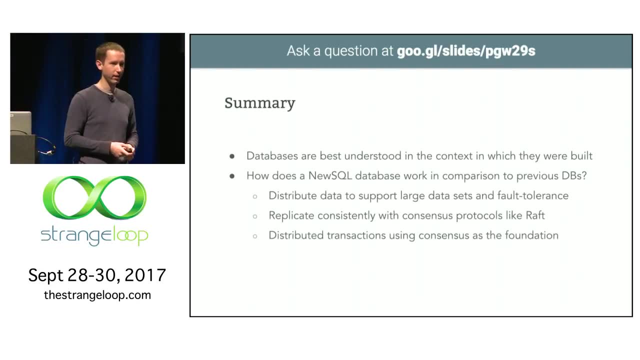 like the MVCC itself and other types of conflicts. So, to summarize, any time you're looking at a new system, whether it's a database or some other kind of thing, you should try to understand why it's being created. How does it fit into the historical context of that type of system? 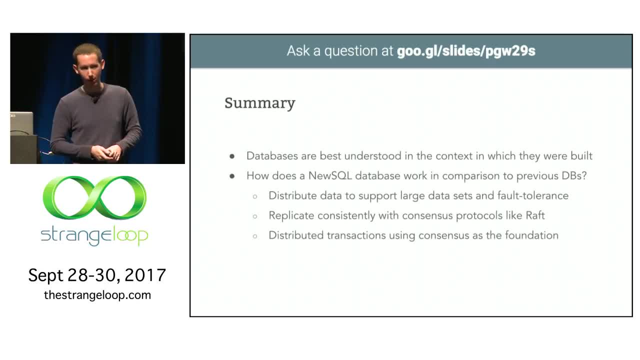 Why is it being built now? Why couldn't it have been built a while ago? or why wasn't it built a while ago? And try to get a better sense for what tradeoffs are involved in picking a system. So we've done that for these distributed SQL databases. 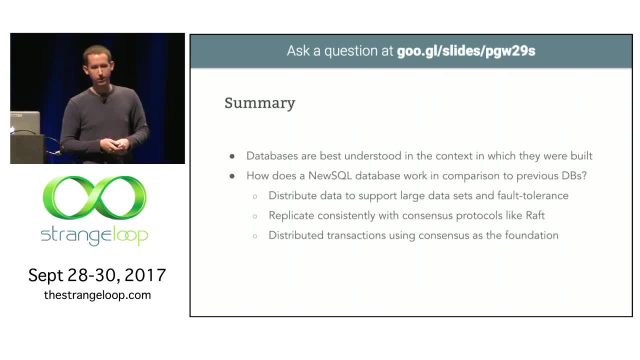 We've also tried to understand how they work in comparison to past databases. So we've done that for these distributed SQL databases. We've also tried to understand how they work in comparison to past databases, So how they distribute data, which they do in a very similar way to these NoSQL systems. 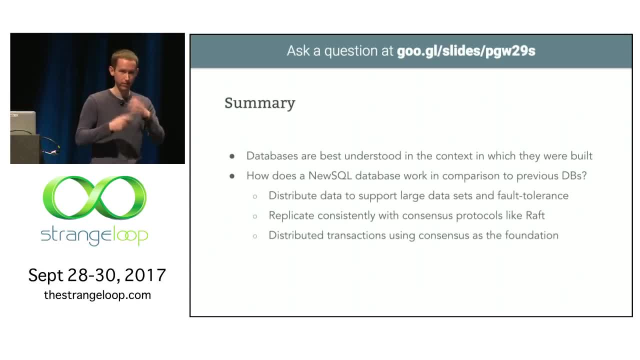 How they replicate that data in a consistent way, which is done in a new way, different from SQL or from NoSQL. It's notably not new to academia, though These consensus protocols have been around for decades, So it's taking this existing work from academia and bringing it into a system in a new novel. 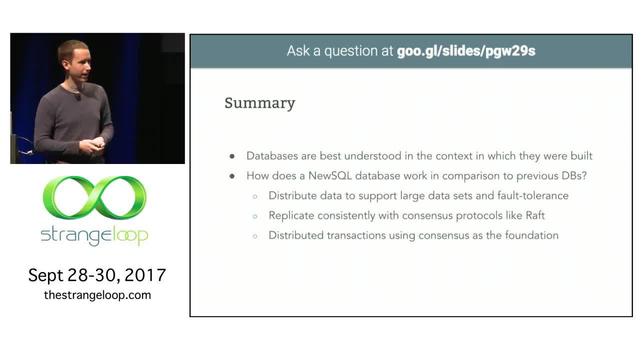 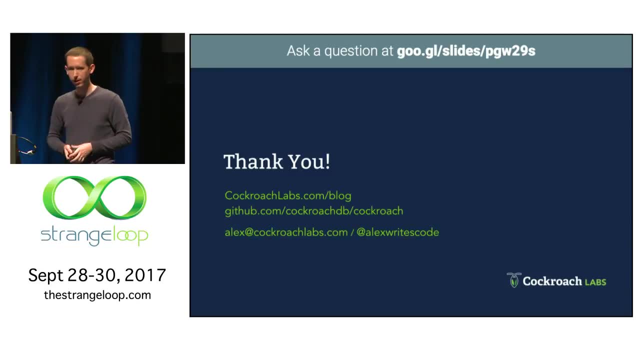 way And then how transactions work, which has been done by learning a lot from how SQL databases work and then just applying some engineering elbow grease to make it work in a distributed setting. So thank you a ton for coming out and listening today. I'll be around for questions afterwards. 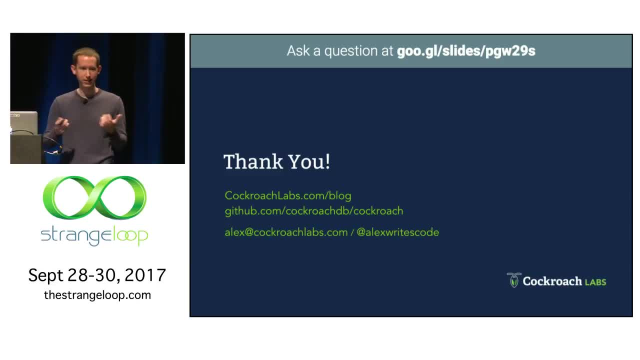 I'd recommend if you are interested in this. there are a lot of great academic papers out there on these topics. You can check stuff out on the Cockroach Labs blog or on our GitHub repository, since it is open source, with all of our design docs. But thank you for coming. 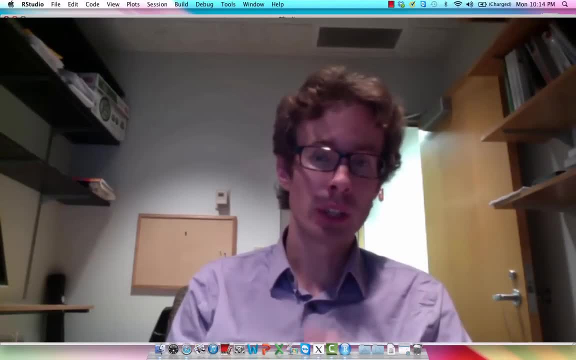 Assuming that you now have R, RStudio and RJags all working in perfect harmony with each other- although in my experience nothing ever works the first time- but for the moment I'm assuming everything is working just fine. Now we're ready to look at some of the example data that comes in. 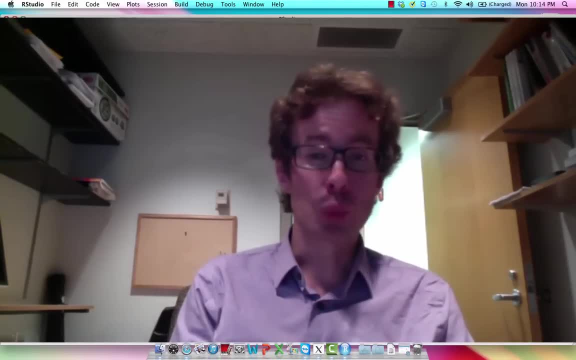 the best folder. After we look at how the inference works in all those different sample data sets. we can then alter it and pretend like we're inserting data from our own experiments and then running it with these programs. So notice, we're going to be using this best example, right? 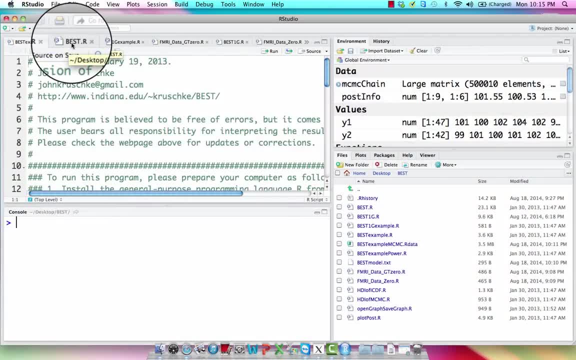 here and remember that it calls upon a lot of the functions in this best folder. Okay, so bestexampler and best1gexampler are basically the equivalent of doing an independent samples in best example and a one sample in best1gexample, ttest. except in this case we're 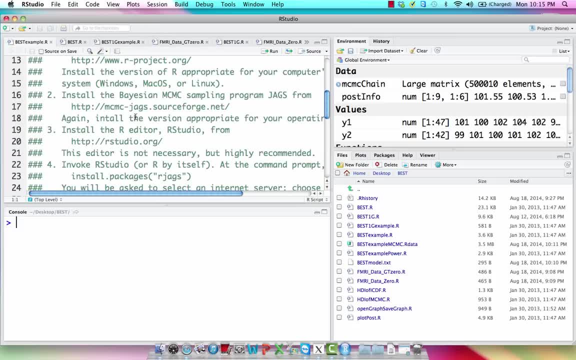 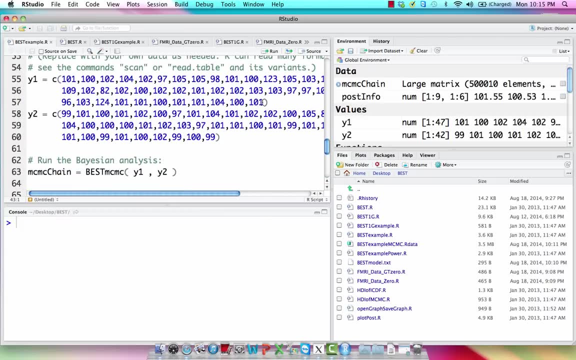 applying Bayesian inference to the data that we've collected. So notice again: a lot of this we're not going to change, but we will change things in these vectors right here. In this case, these are just placeholders, surrogates for data that you would collect. 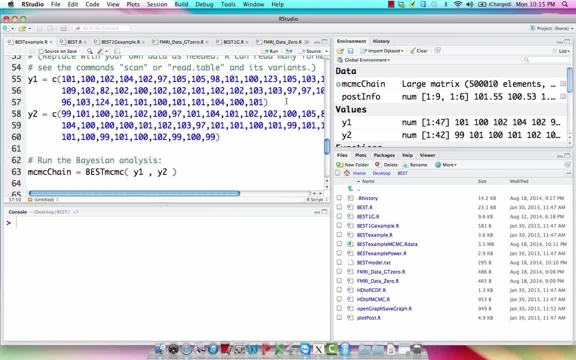 in the actual world. Now here's this kind of arbitrary data to illustrate some of the properties of Bayesian inference. So in this case you would simply replace all these values with the values you collect. It could be behavioral reaction times, it could be percent signal change in an. 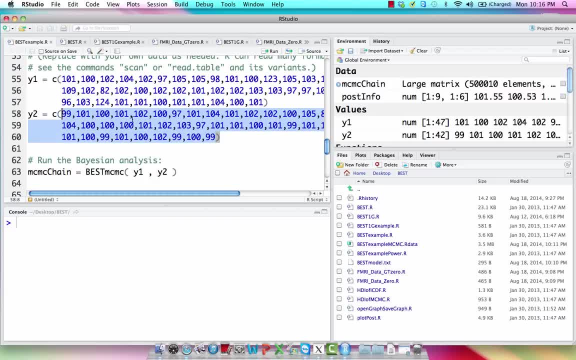 fMRI study and you would just put that in the best example. So now we're going to look at the Bayesian inference. So we're going to put them in here, separate them with a comma and then run the program and it would call upon all the appropriate methods and functions to run Bayesian. 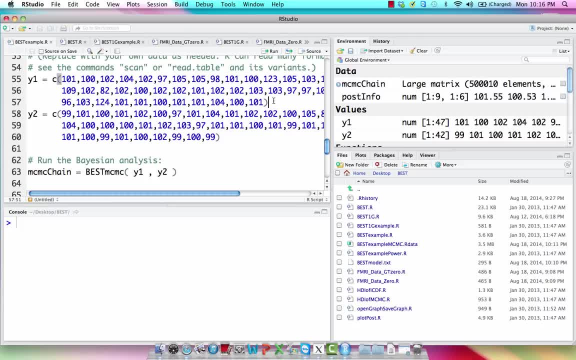 inference on your study. It really is as simple as that. If you want to again make this more custom and change some things to suit your own evil purposes, you can do that by altering some of the code in the rest of these folders right here, specifically bestr- best1gexampler.